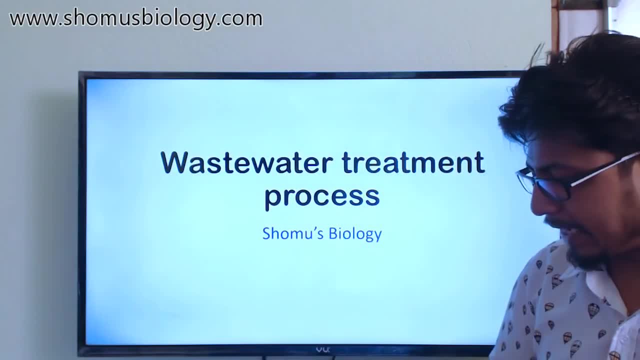 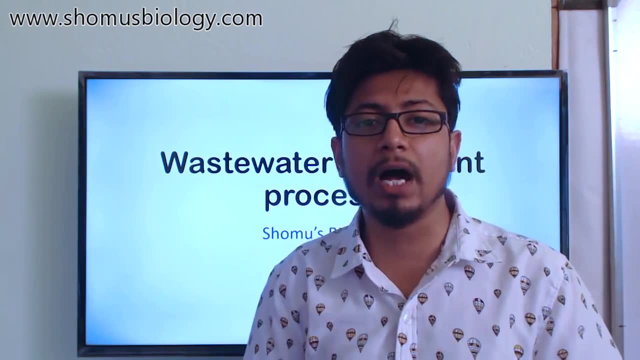 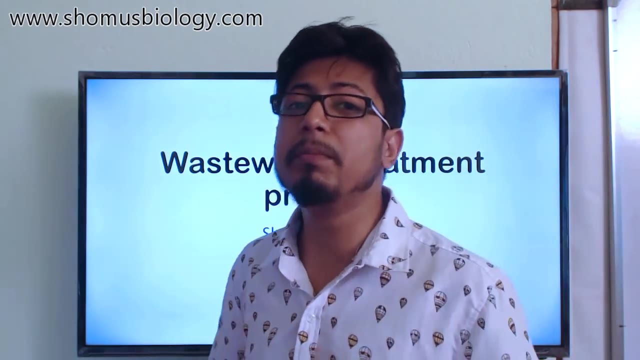 treatment in a typical wastewater treatment plant. there are different types of wastewater treatment plants with modified versions of different steps, but overall the general out of the view is the same. so in this first video it's about the overview of wastewater treatment and what we mean by this wastewater. 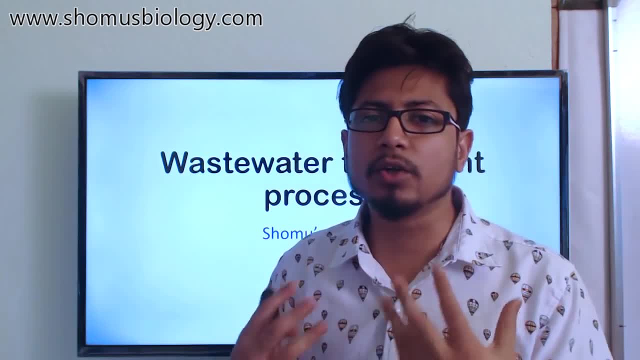 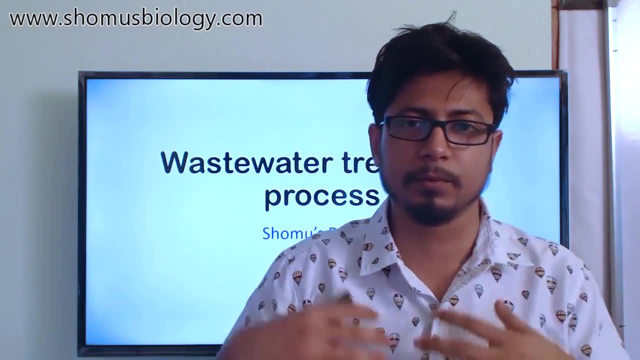 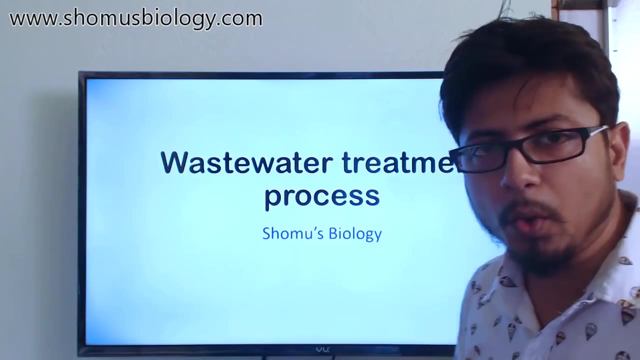 treatment. now. by this time i already told you that it's about the raw sewage, that we have used, the excess amount of water that is the leftover after we we bath, after we flush down the toilet. now that amount of water is finally transported from our home to a sewage treatment plant or a wastewater treatment plant. 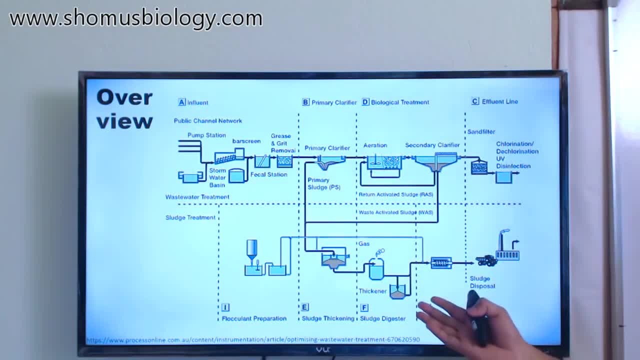 and what happens in that wastewater treatment plant is this. now, when you look at this picture, it feels really, really uncomfortable, because a lot of different components, a lot of different techniques and machines are drawing a schematic drawing in this particular picture. so first, what we will talk about. we'll talk about: 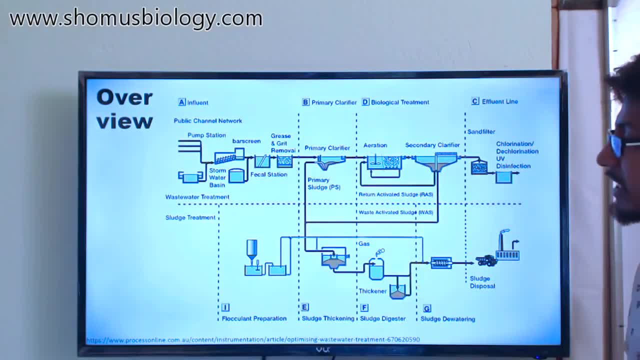 all of this setup and what are the sequence and stages of all this process. and then we'll talk about each of these different steps of wastewater treatment processing in much more details in a separate video. so in this video i'm just going to talk about the overview. now, if you look at 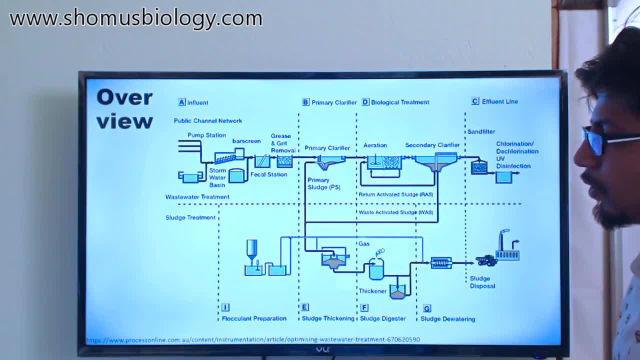 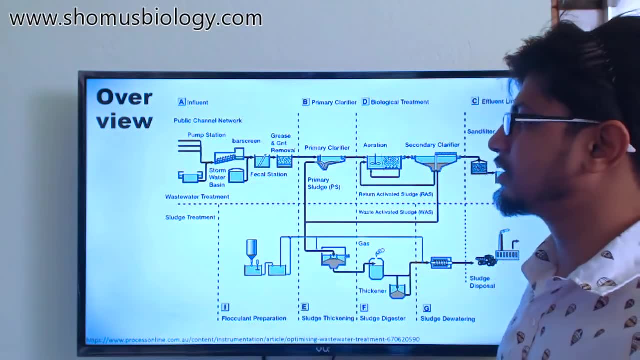 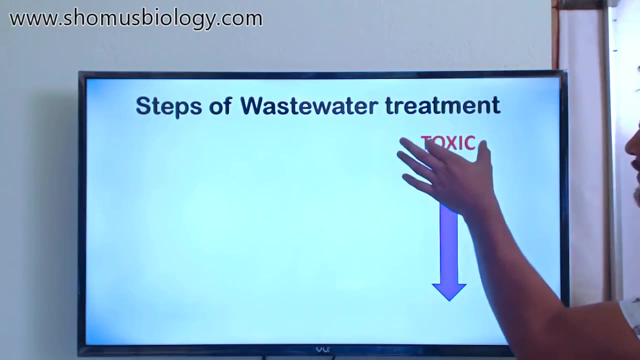 this picture it finds really, really complicated. but before going in there, let me tell you the steps of this wastewater treatment. then i come back here in this picture and explain how these steps actually work. now the steps of wastewater treatment are the following: so the wastewater treatment begins from the toxic part of the water and 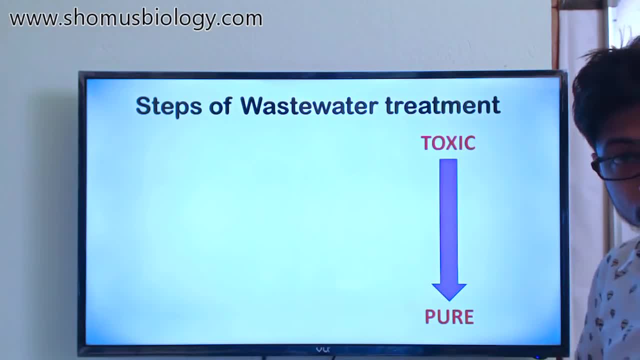 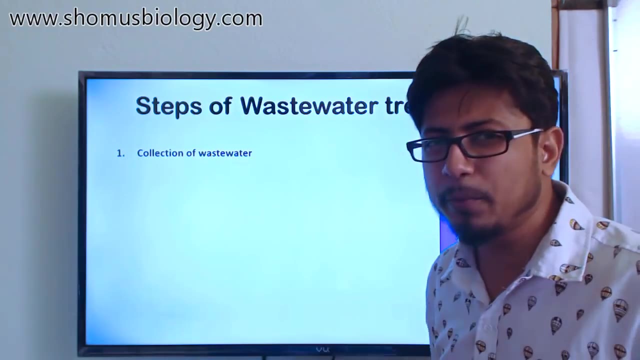 then it finally goes towards the pure water that we can use for domestic purpose, the portable water, as well as sometimes the water that we can even drink. so the journey from toxic water to pure water, it begins of the collection of wastewater. that's the very first step. 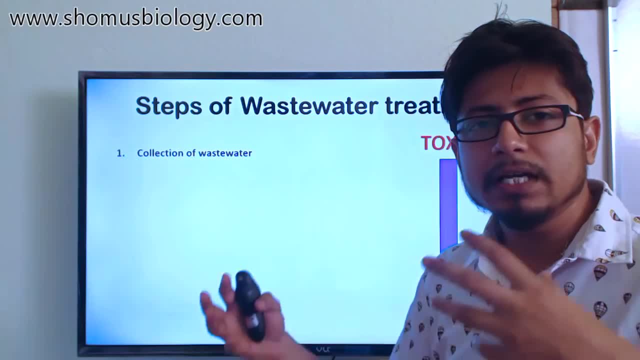 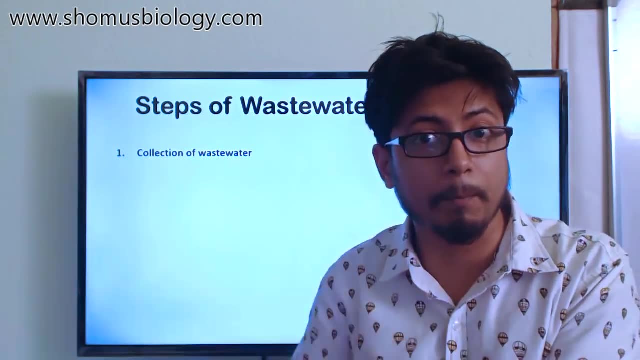 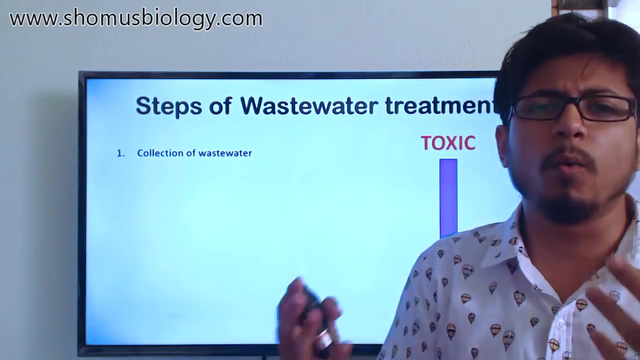 collecting all the wastewater from every single household in a neighborhood and from out of every single home are collected by huge collection pipes. those pipes are generally made up with iron or concrete. generally these pipes are not visible, so you cannot see that why we fail to see this kind of pipes. actually they are. 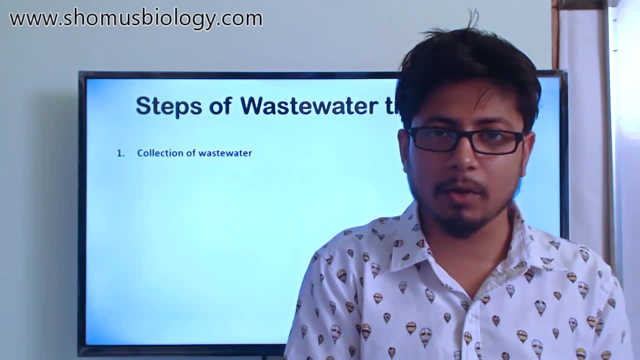 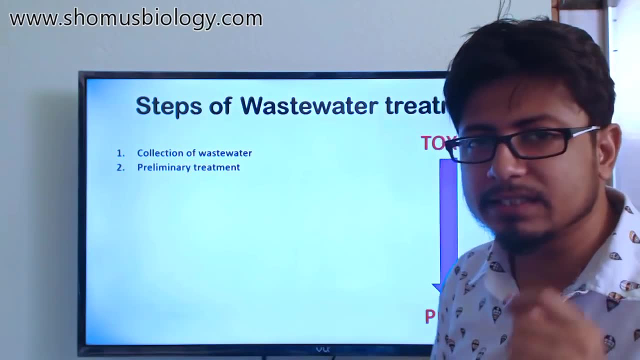 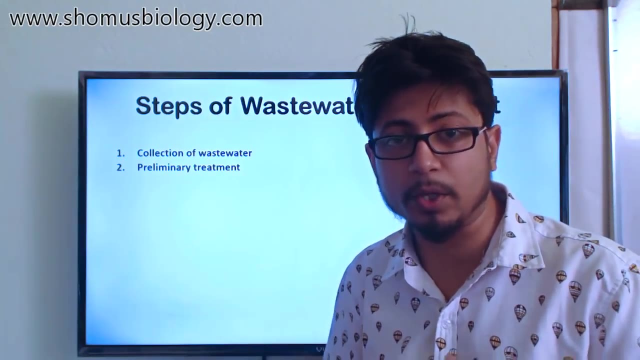 present below the ground so you cannot see this, uh, all the time. in few occasions you can see, but most of the time this is underground pipes are collecting all the wastewater and then the step cause: preliminary treatment of wastewater. so when you say the different modifications of wastewater, we call it. 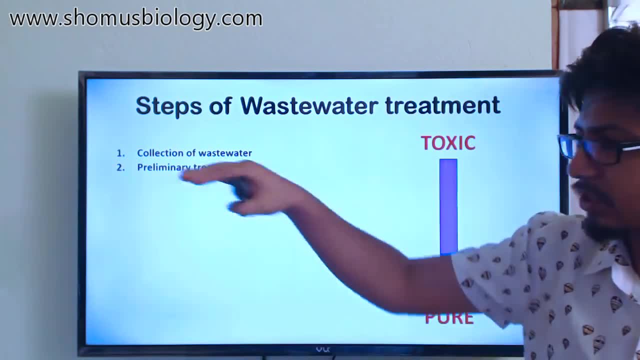 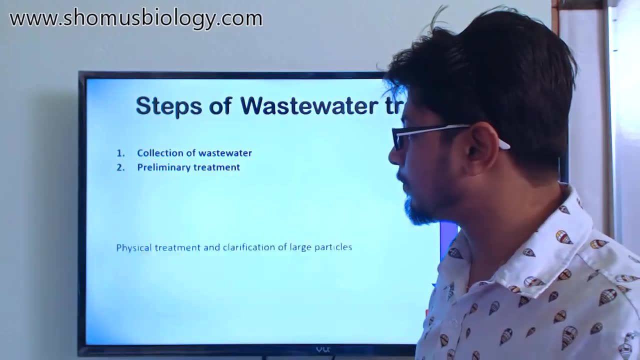 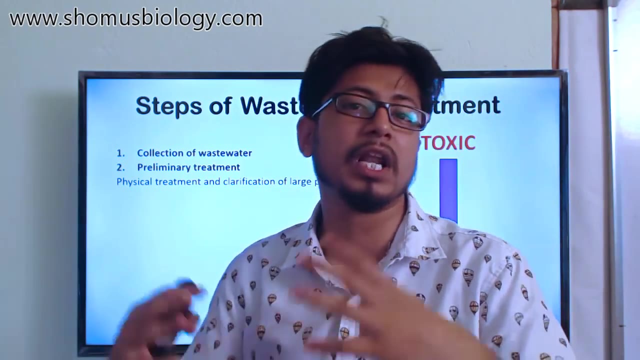 as treatments of wastewater. so preliminary treatment is a starter treatment process. in a preliminary treatment of wastewater what happens is that simple physical uh change. this is a physical treatment and clarification of the wastewater, of generally, the clarification of the large particles, so the wastewater that we have it carries. 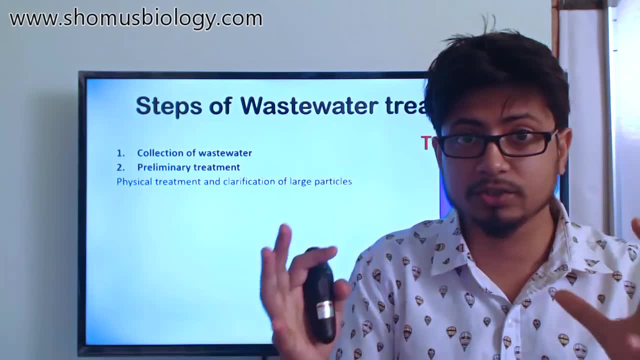 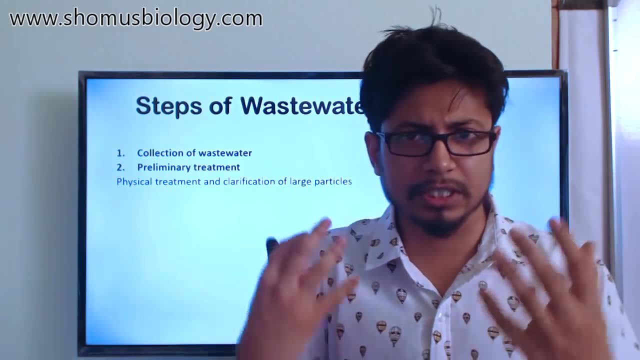 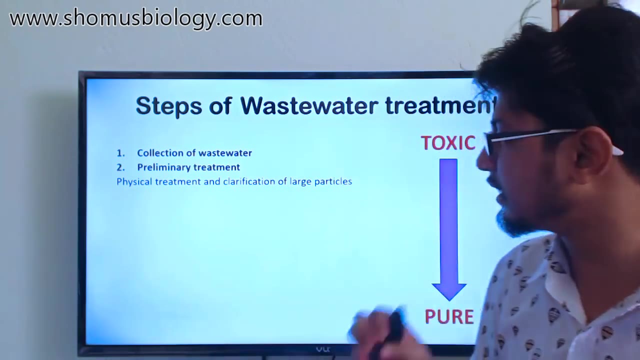 many impurities. it carries all the solid particles: large solid particles, small solid particles, solid particles. it includes all the organic matters from the wastes that carry nitrogen, carbon, sulfur, phosphorus, organic wastes. along with that, uh, it also carries some chemical waste, so all these things are present in that wastewater. this preliminary 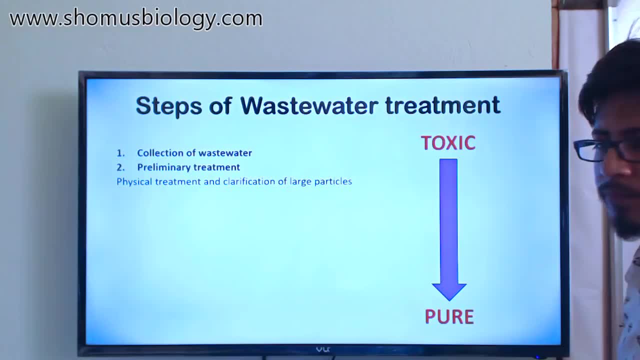 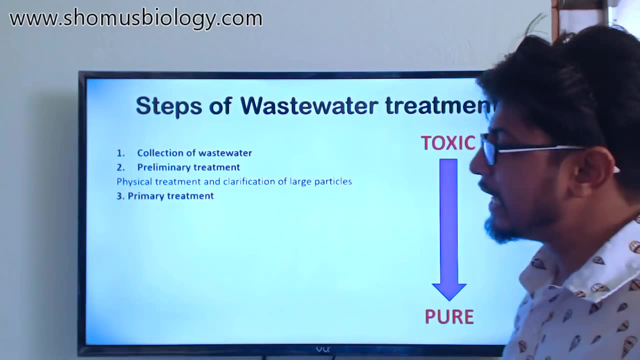 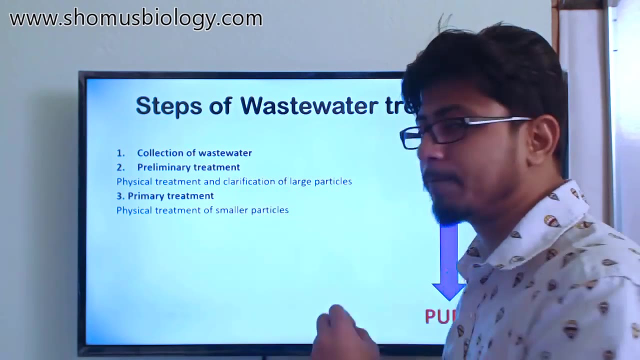 treatment is designed to only separate the large particles uh from that wastewater. then it converts through the process known as primary wastewater treatment. in the primary wastewater treatment it's also physical treatment of physical separation, but a physical separation of smaller uh particles compared to the preliminary, because in preliminary we are separating. 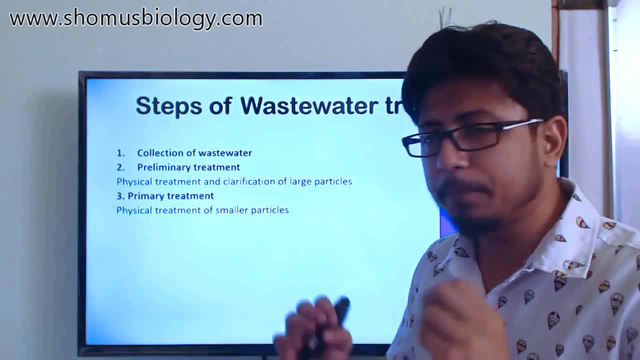 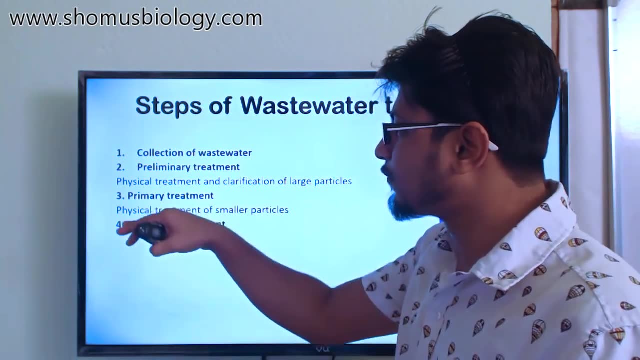 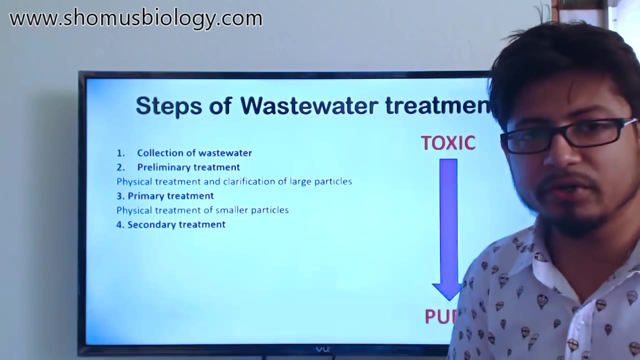 the large particles with screeners, giant screeners. but in primary treatment we're separating small particles and then afterwards we have secondary wastewater treatment. so after the preliminary primary treatment all the physical measures are there. uh, separation of solids from the liquids are done. so in the secondary treatments. 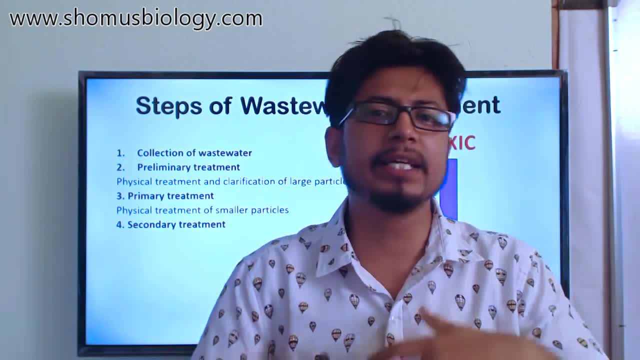 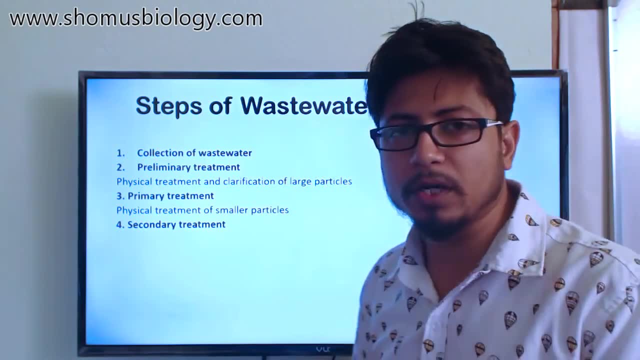 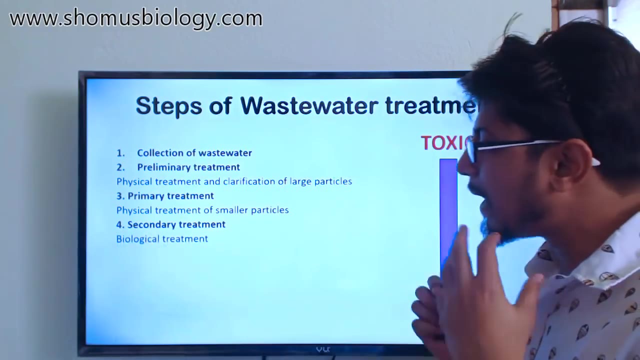 we mostly have liquid waste water. they don't carry any small particles because those are already removed by preliminary and primary wastewater treatment. so in secondary wastewater treatment we use biological agents like bacteria, fungi or protozoa, and this biological treatment kind of causes to take out all those organic components that are present in 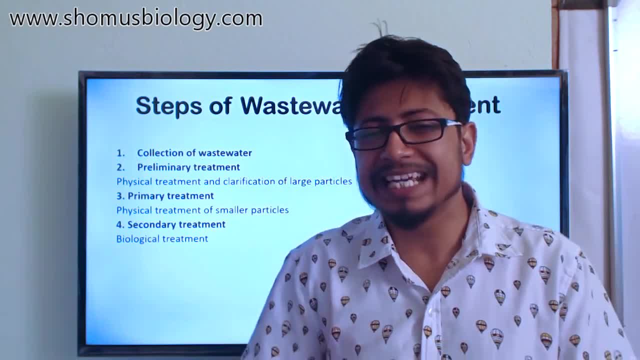 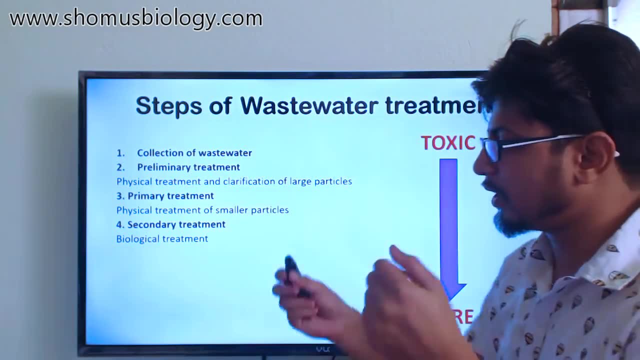 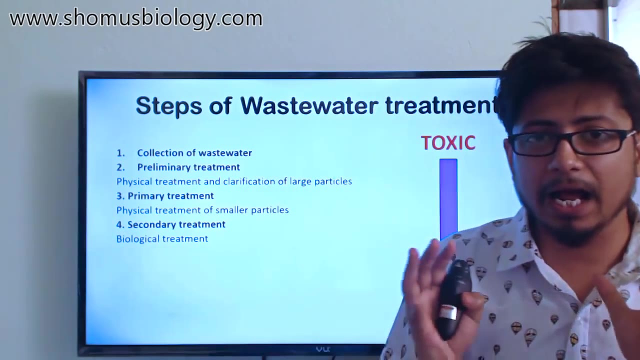 the water and they use those organic components to grow themselves. in turn, they're reducing the amount of organic compounds in the wastewater, and that is really, really important. we call it secondary wastewater treatment. so after the secondary wastewater treatment is done, so in secondary wastewater treatment we- uh intentionally add microorganisms in huge chambers where this liquid 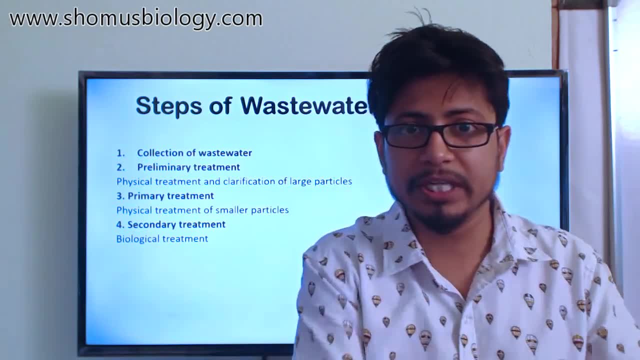 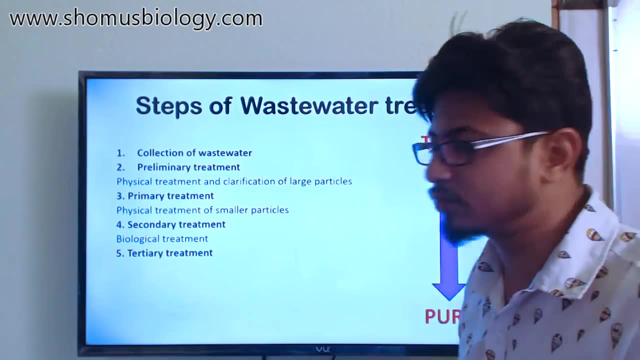 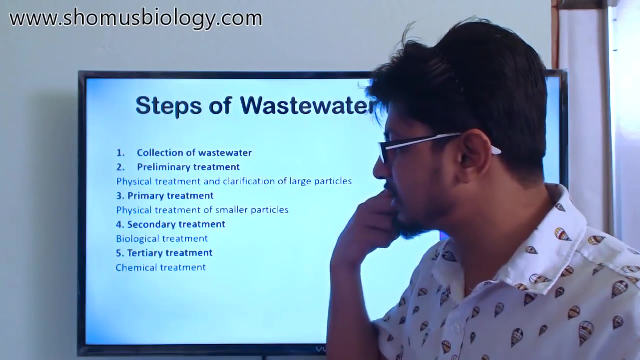 wastewater is present so that those organisms can do their job of eating all those organic compounds, and that's really, really important. then comes down to tertiary treatment. the tertiary wastewater treatment uh comes after the secondary treatment. in tertiary treatment is the chemical treatment process. chemical treatment means, you know, in 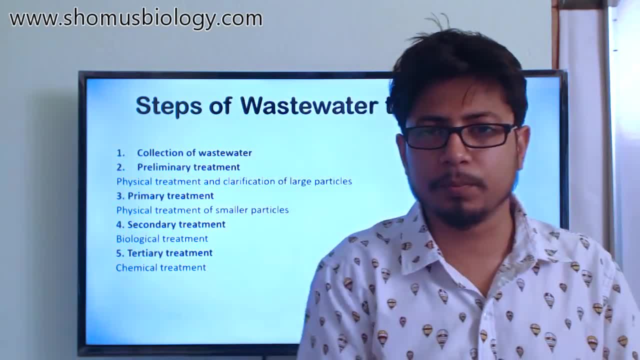 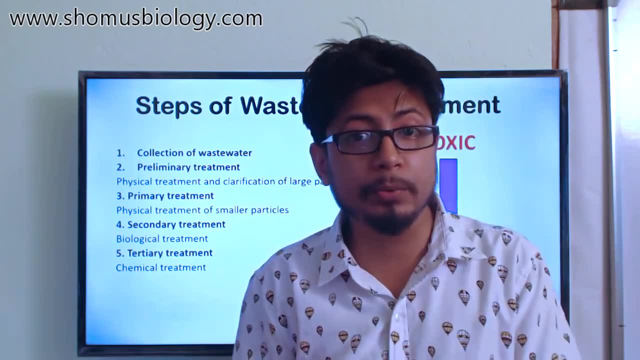 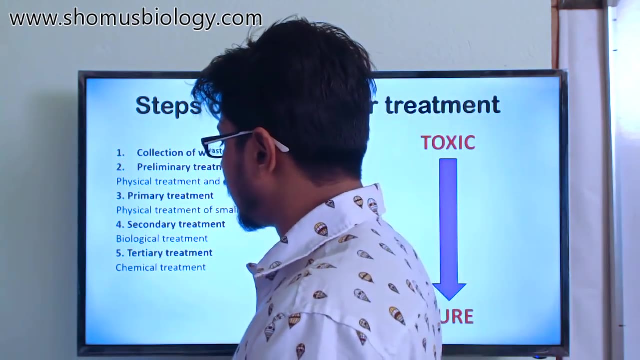 this case, we simply use chemical agents, uh, to pure or purify the water. example of this chemical agents are ozone gas or chlorine as a gaseous form, liquid form or solid form. we can use sand filters. we can use reverse osmosis, so there are many different uh mechanisms used. 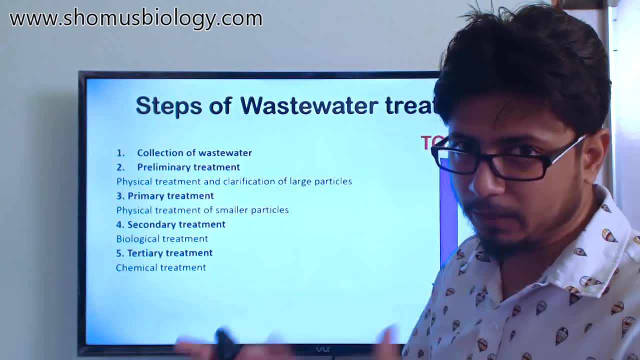 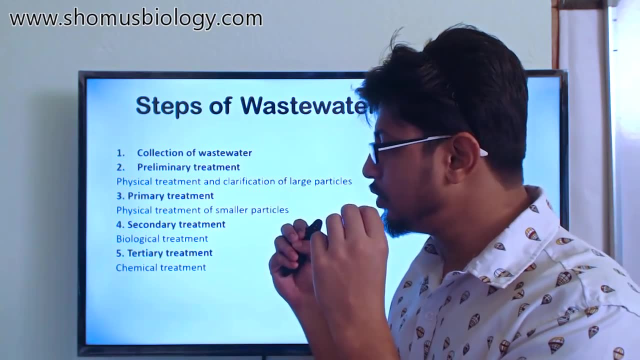 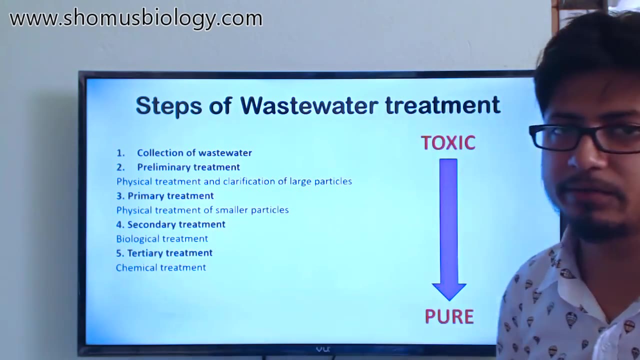 uh to purify a water. so we generally use this chemical treatment, like chlorine ozone uh for treating uh this, this wastewater, at its scent and generally we use this chemical treatment uh to reduce the odor as well as to kill any of the present microorganisms that we use in the secondary treatment. because you know, 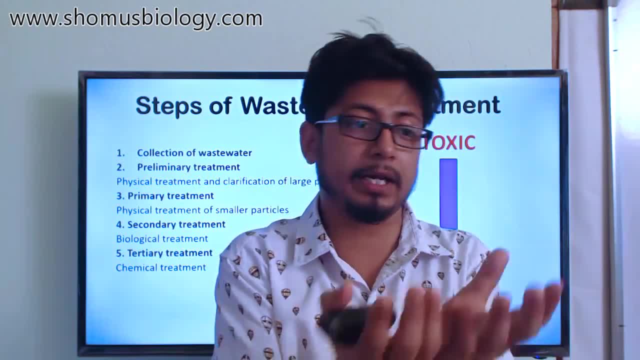 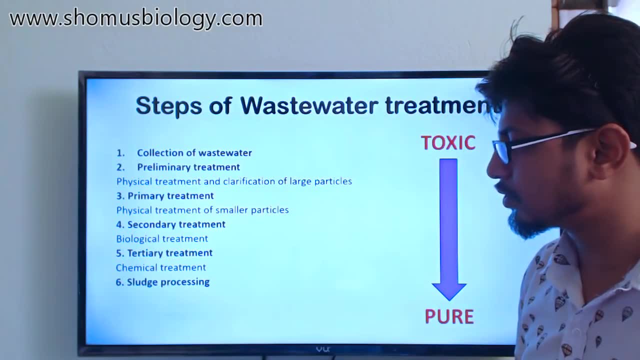 you cannot put microorganisms, bacteria and fungi in your water, and if people drink it they will feel sick, so that's another thing. so you need to kill them with these agents. and then finally, it comes down to sludge processing, because till this point we are talking. 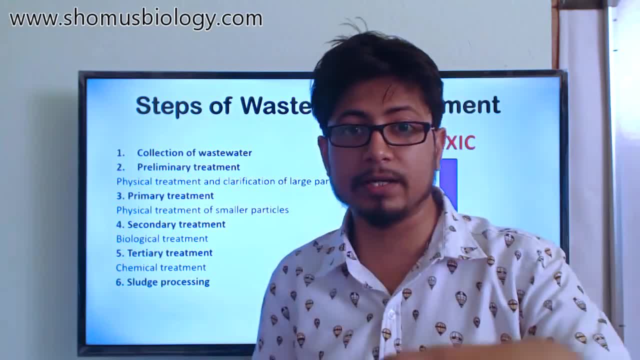 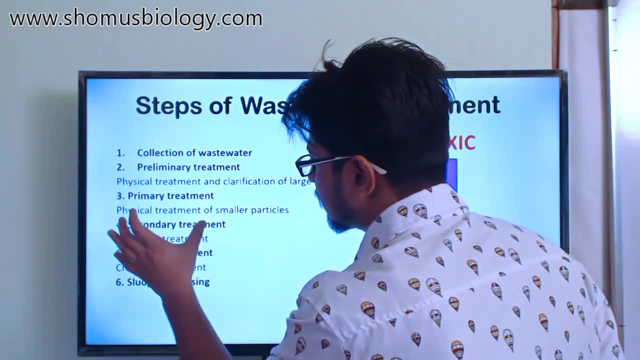 about on the liquid part of the water. so water comes in from one side, known as influent, and goes out from one end, known as effluent. so this process continues now in every single steps, like uh, this primary treatment, secondary treatment. in all these primary and secondary treatments the water is treated either. 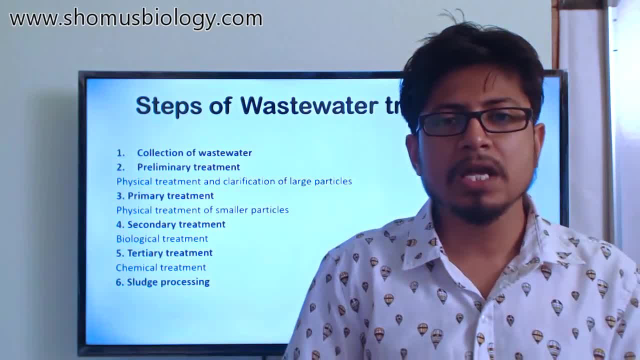 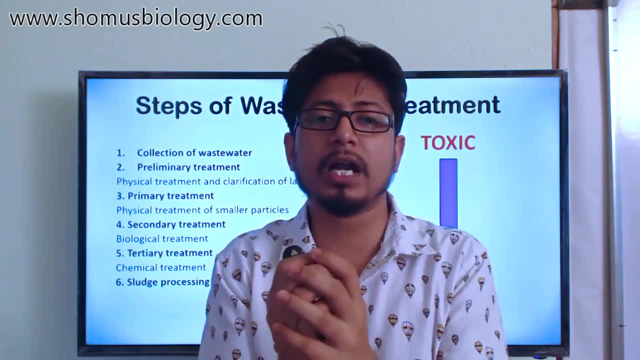 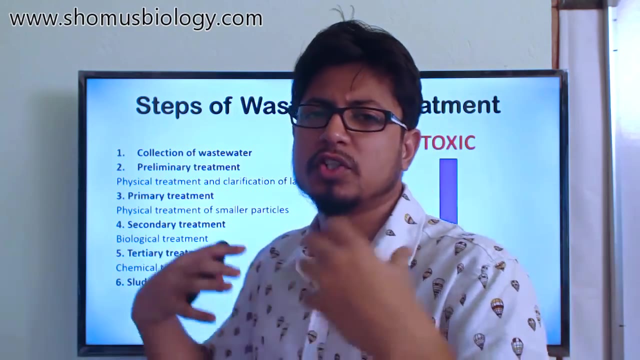 physically or it's treated with biological agents. but at the end the water is transferred to the next round and the, the components, which are particles and float components, start to form flow, and flow of this, these components, matters, are condensed and they settle down to the bottom of those large giant tanks known as clarifiers. primary 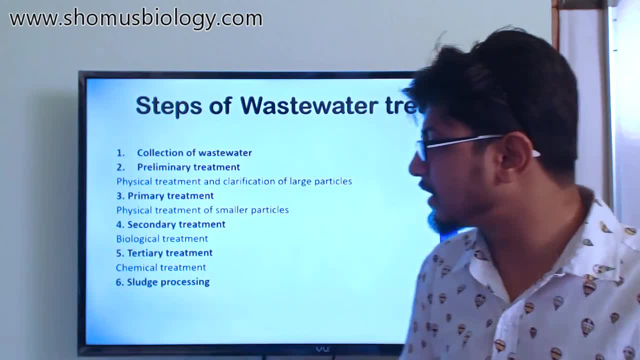 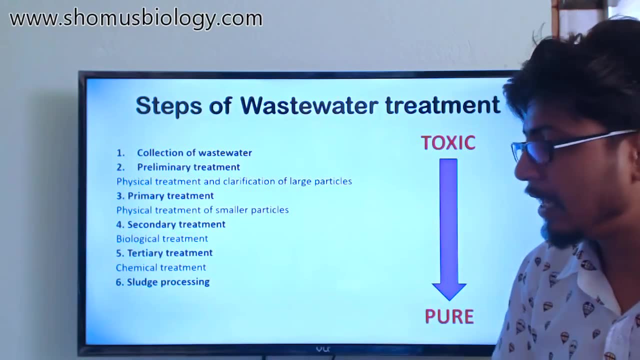 sedimentation tank, secondary sedimentation tank. primary sedimentation tank is when we use the primary treatment, secondary clarification or secondary segmentation tank which we use in the secondary treatment. so at the end of this primary and secondary treatment we have all those, all those components settled down to the 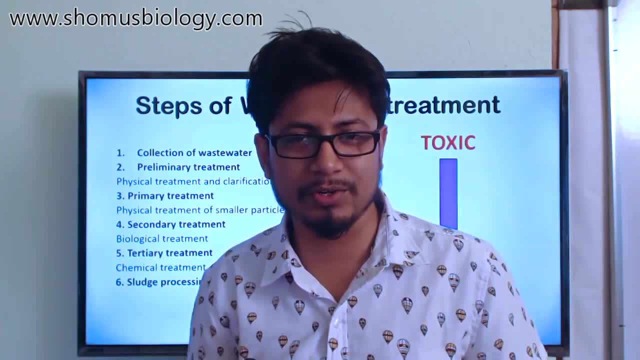 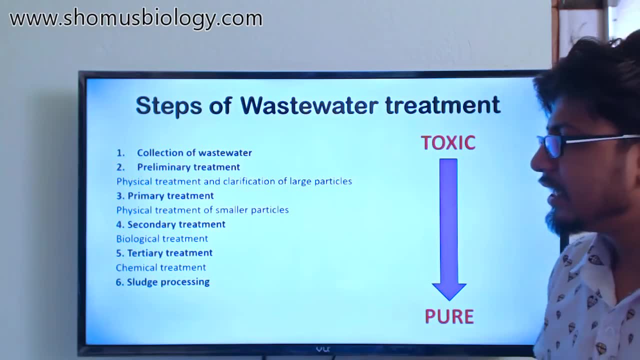 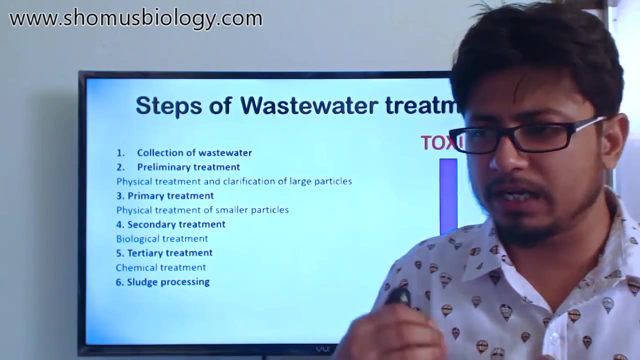 bottom of the tank. we call it solids of wastewater. treatment and handling of the solids are known as solid handling part and we can also call it sludge. so sludge is anything which was present in this wastewater, which is the decomposed part of the organics, as well as the bacterial dates: uh, dead. 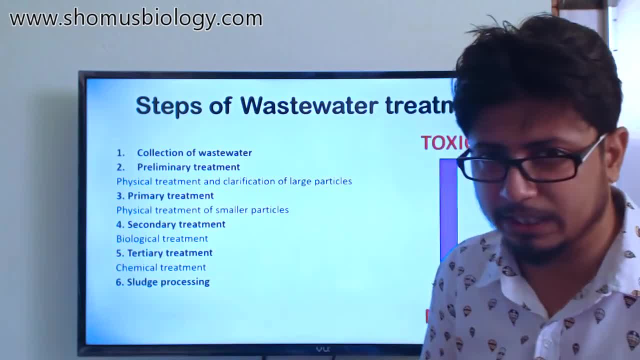 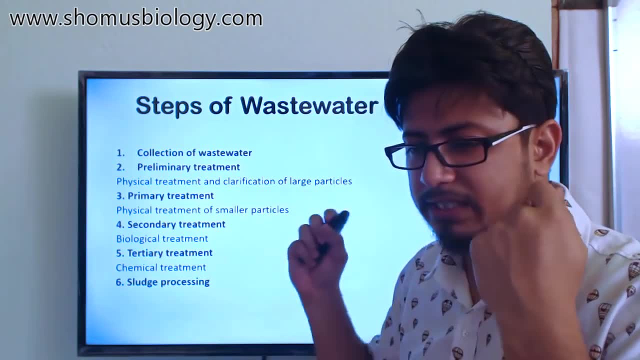 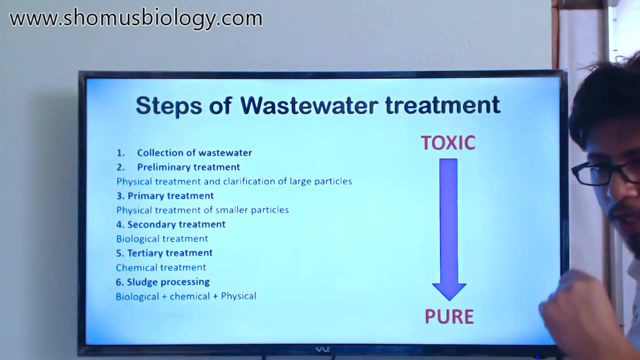 cells, bacteria, fungi, all those things which were used to treat in the secondary treatment, everything as a particle matter that we can see, it can settle down. so you take all the sludge and we process the sludge. sludge processing involves three different types of treatment together: biological, chemical as well as physical treatment. 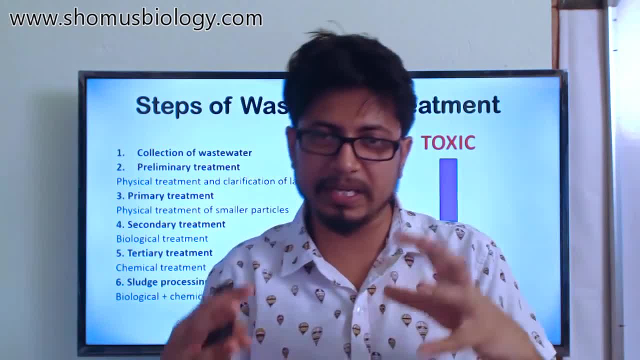 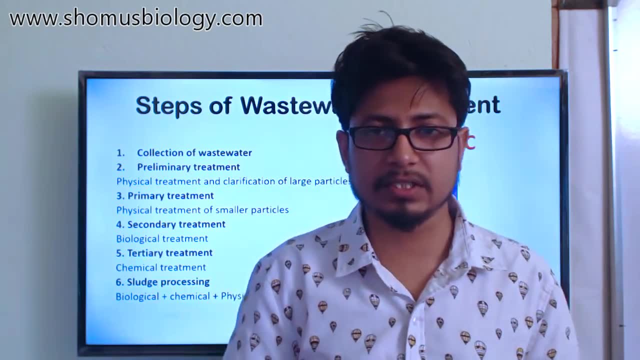 we, we generally uh condense the sludge to make it thick. so thickening of the sludge, then digestion of the sludge by heating it and then finally dehydrating the sludge gives us very compact portions of the sludge, which is also filled with some major nutrients. 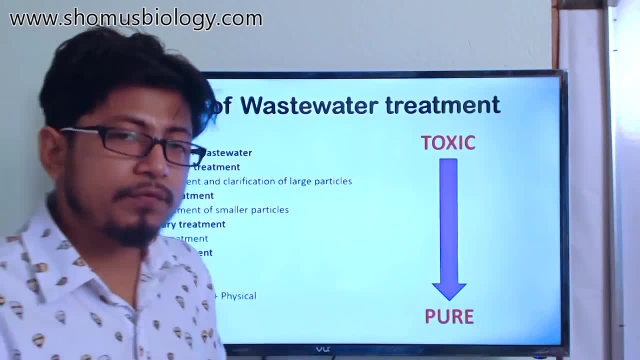 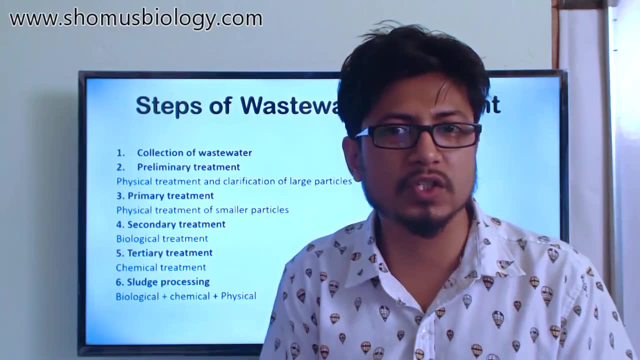 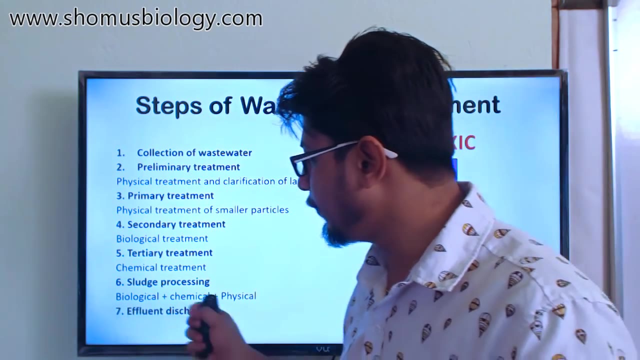 and organic compounds that are being derived from the wastewater that came in at the very first place. so we can use this sludge, uh, to increase the fertility of the soil. so that's what it means in the land fields in agricultural purpose. okay, so these are the steps and finally, if we went to the 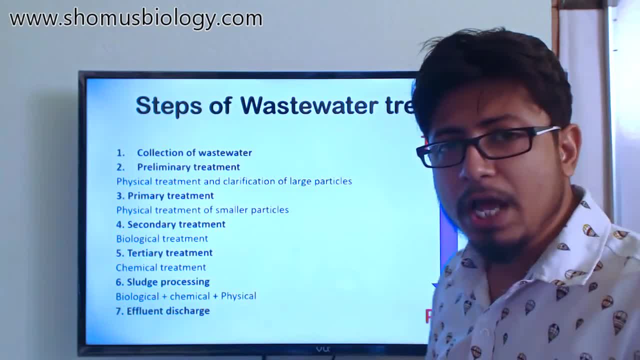 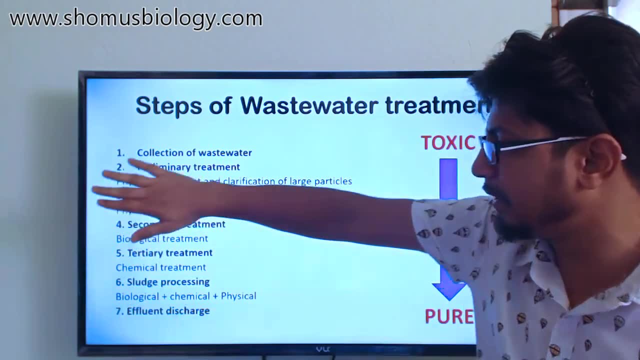 countryside to make a sludge. they would bring in this water and water would also come in this liquid which would then get into the soil. so it would take the sludge and then every year we take off the sludge to the soil for a year and now the sludge is gonna come in. 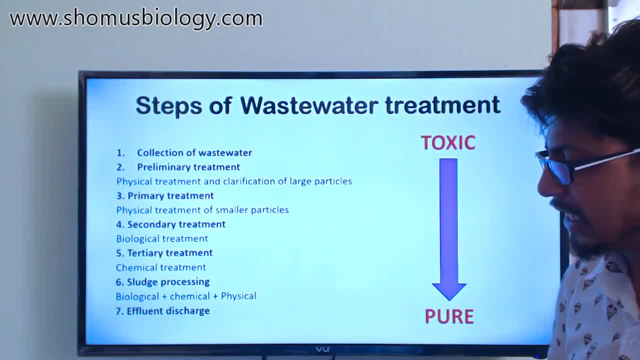 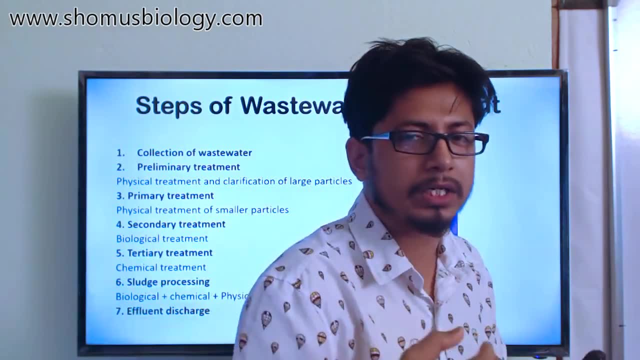 the soil of our house which we're gonna want to use for our household health. so that's later on. we will take our sludge and take it out of the soil and we will mix the water with the sludge, and so here we have the sludge and we will use this sludge to apply. 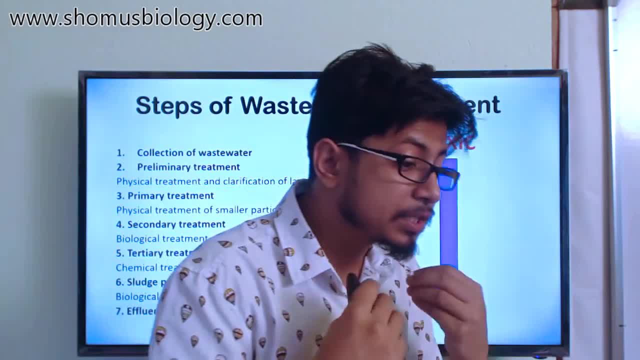 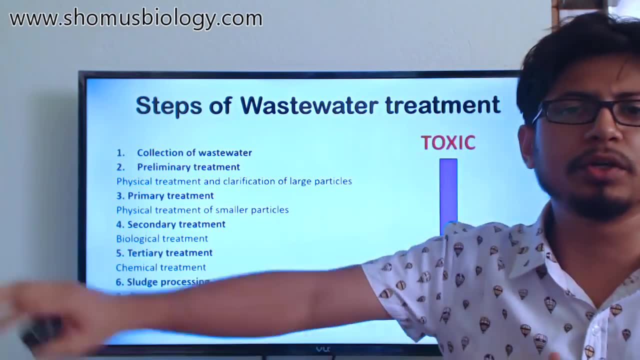 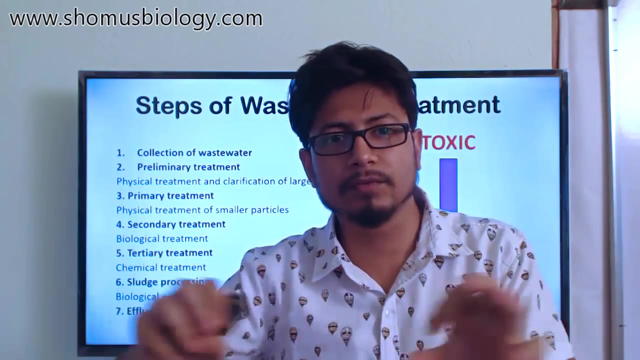 drinking. but for drinking we need to add some more safety, some more additional advanced tertiary or chemical treatment, even after the tertiary treatment. so sometimes you know invincible corporations, what they do when the water comes in. they also ingest chlorine in the, in this pipe of the water supply. so 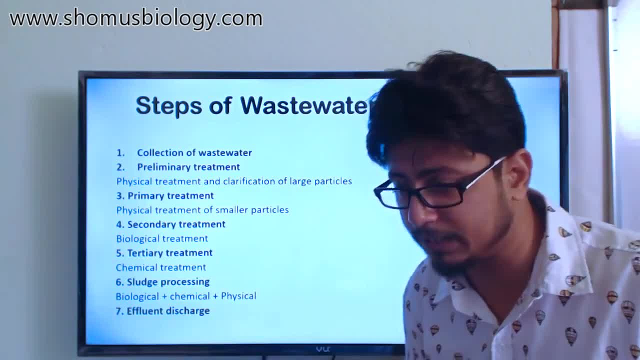 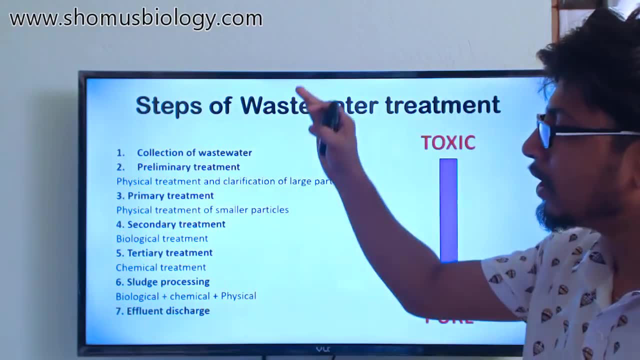 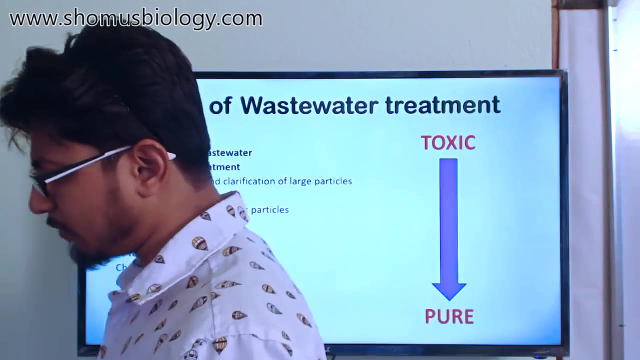 that any further contaminants can be killed, even if anything remains in it, but still definitely that we can produce. going through all the steps, with a proper quality control of the specific waste water treatment plant, we can produce pretty good quality effluent coming from a very harsh and toxic 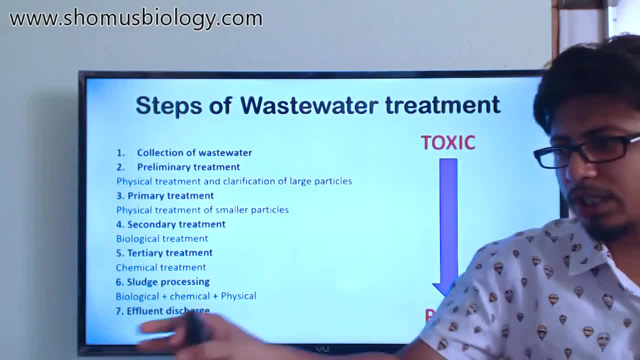 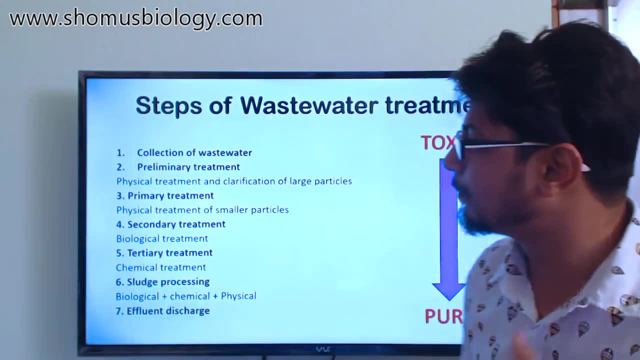 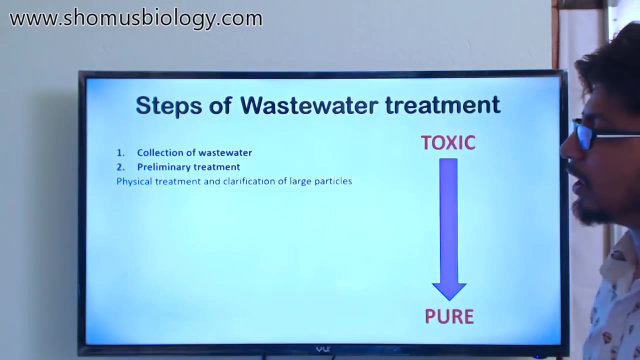 sewage. so that's what we can do. a sewage that you just flush can come again in your shower and easily use it, and even you can drink that water with the help of the steps of wastewater treatment. so now, if I go back and show you the picture here, 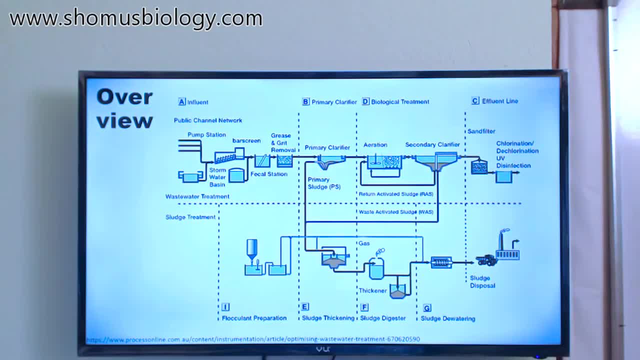 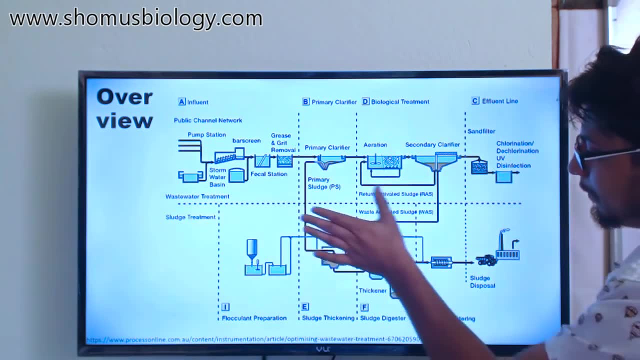 you'll understand what we're talking about now. this picture explains two things, you know. one is this dotted line separating few steps from the other. now, anything bottom of this dot line is the sludge processing or the solid handling, and anything on the above is effluent handling, just water handling. so it 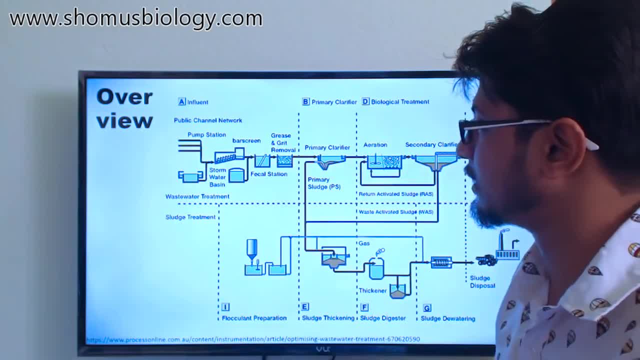 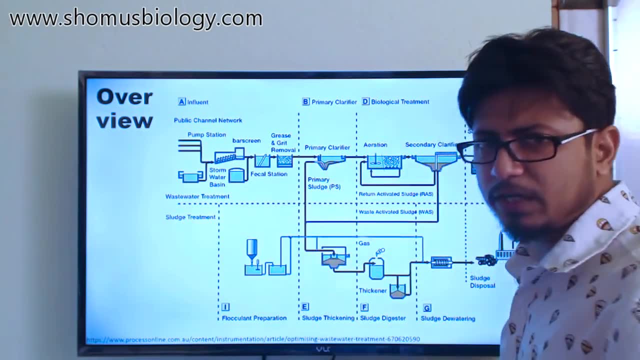 begins with this: the pump station. they're collecting all those sewage and finally they're transferring to the preliminary treatment. so this is the preliminary portions of the treatment where it involves the water and the water, and when you look at this you'll see that it involves several. 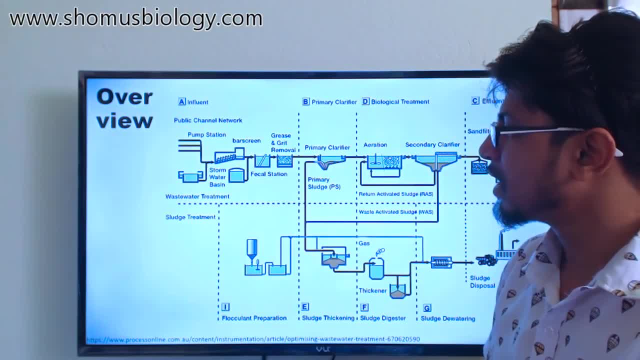 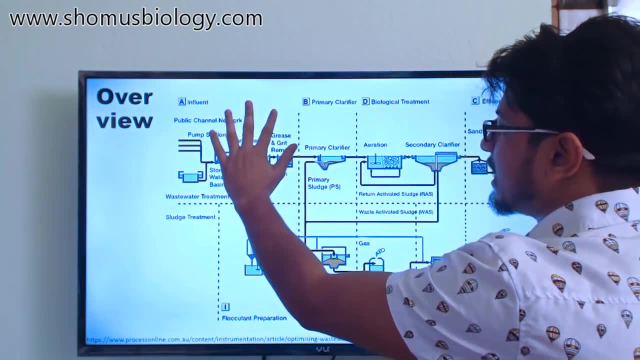 different screeners, giant screeners with separate large particles from the water as well as a grit chambers where settled down. so those grit and small ripples, the separate those things out at this point: preliminary treatment. then the water is transferred to the primary treatment and you can see in the primary 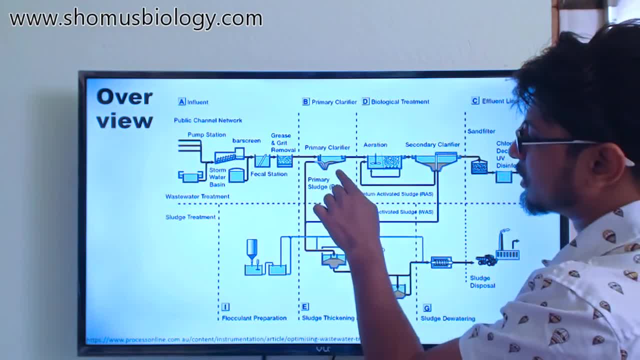 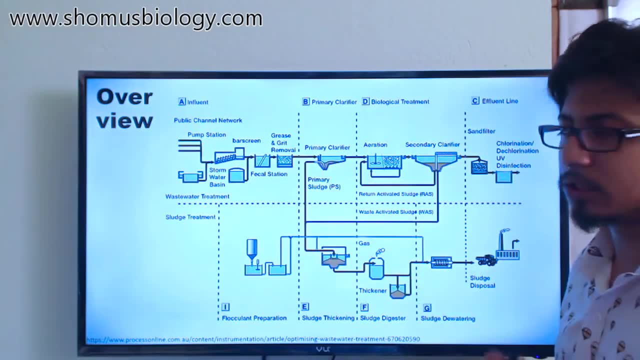 treatment. we have the primary clarifier or primary sedimentation tank. so, as you can see in this picture here, blue color means the water as well as yellowish- twice through this process, always for the treatment: one is during the primary clarifier settlement, second during the secondary clarifier settlement. so this 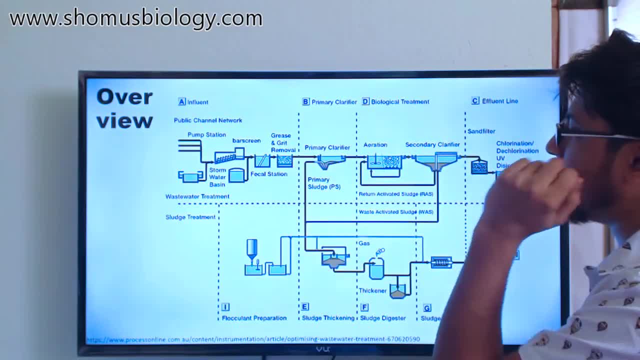 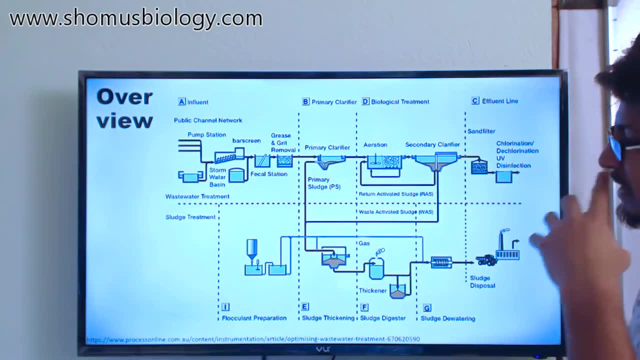 is where the sludge is produced and then the water is transported to the biological treatment. in a biological treatment what is done is aeration and after the aeration, you know, microorganisms are added, they start doing the job and in the secondary clarifier, again settlement of the sludge water is. 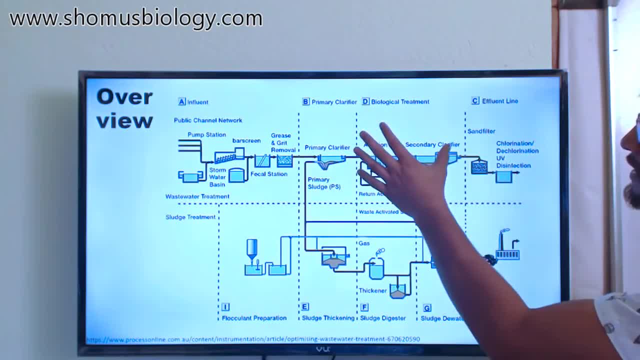 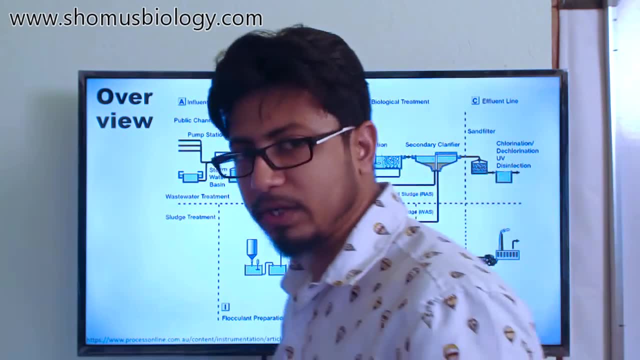 present on top, and then again water start to move out there from the secondary, worst water treatment to finally to the effluent discharge center and this is also known as the effluent purification or effluent clarification, because this is also known as the tertiary treatment or chemical treatment. so this is 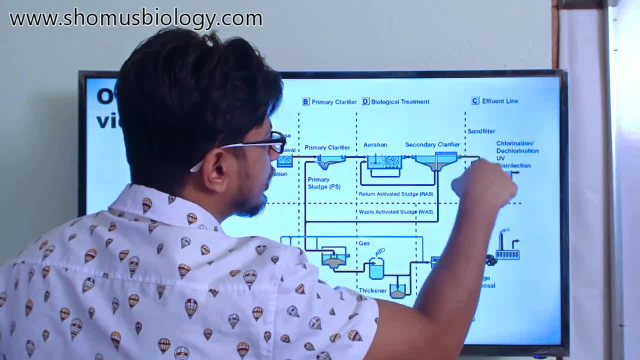 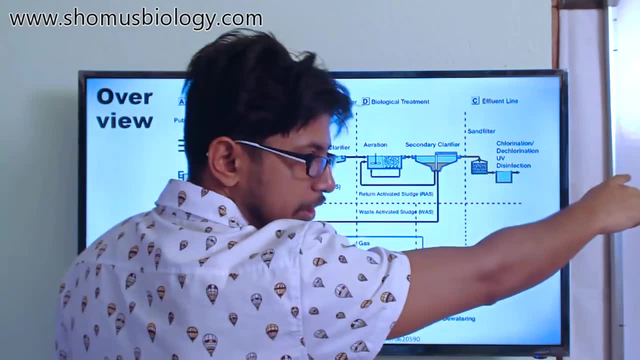 preliminary, primary, secondary and now tertiary. in the tertiary treatment you can see coordination, UV and disinfection of the effluent is done and then the effluent is discharged finally. but what happens to the sludge? because we know sludge is produced in the primary and secondary water treatment and then the effluent is. 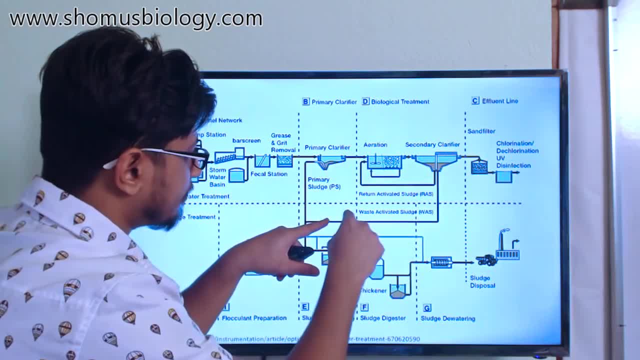 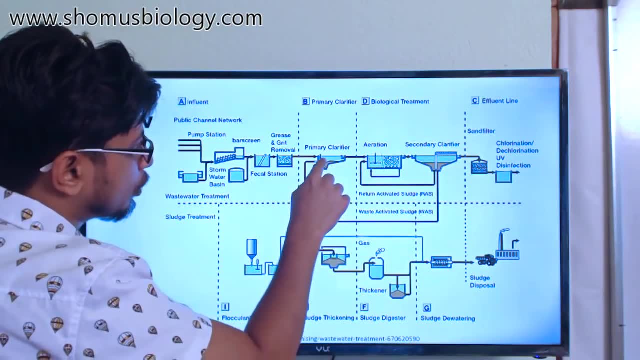 collected from the primary clarifier as well as the secondary clarifier and that sludge is taken right. generally, the sludge produced in the secondary clarifier again takes a journey and it's collected back and pushed into the primary clarifier so that it can take the 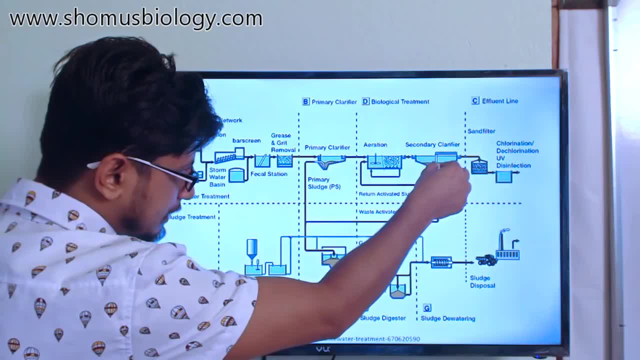 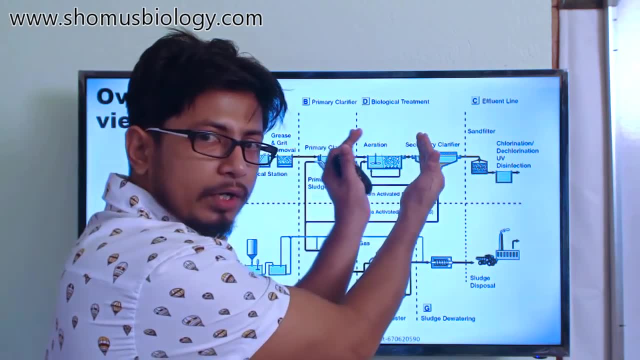 journey again, so it's a repeated cycle. the sludge produced in the secondary clarifier goes back to the primary clarifier and then again takes the journey as much as times it's possible, because this is where the microorganisms are working, and not always microorganisms are utilizing. all the these are organic matter in the 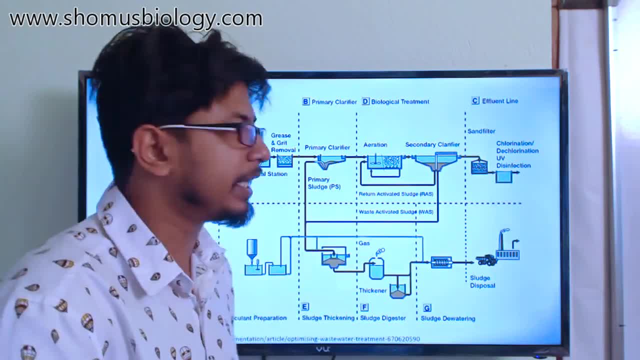 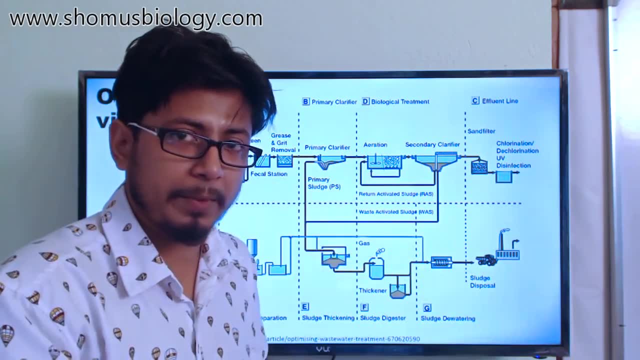 in the water and in the sludge. so we keep on repeating sludge so that it kind of help to feed the microorganism because we're not transporting or adding something from outside as a as a food for microorganisms. it's all about the sludge and sludge materials, what is eaten by the microorganisms. so this: 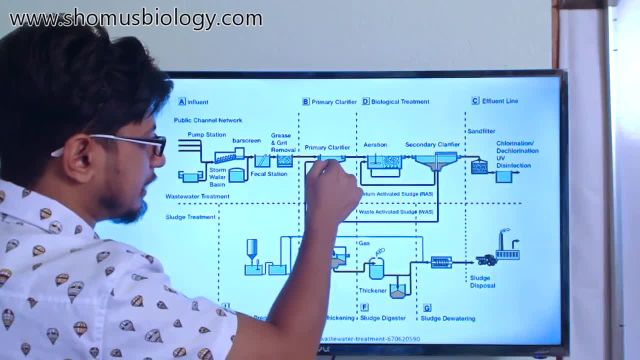 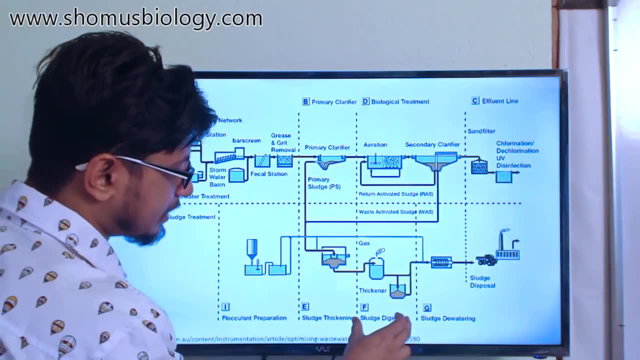 process keeps on repeating there. but ultimately, once this process done, the sludge is collected and the sludge processing begins where it occurs. three different stage: sludge thickening, first step. second stage, sludge digestion: by heating the sludge makes an increase the water content, and then again 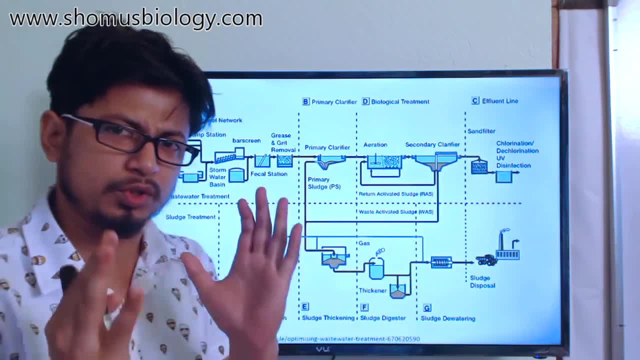 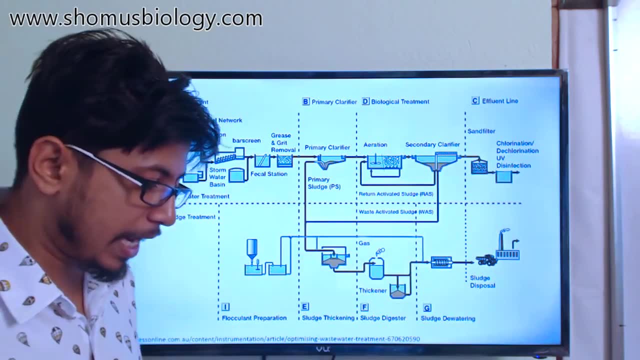 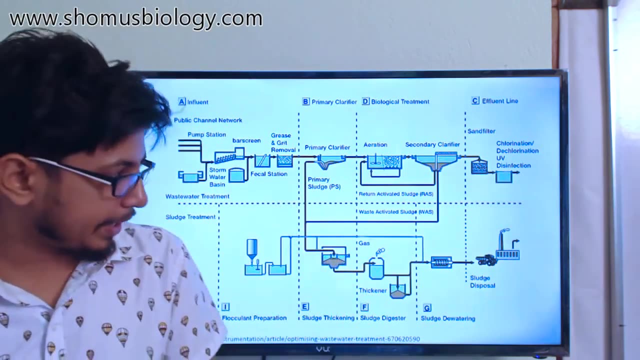 dewateration or dehydration of the sludge to produce solid cakes of sludge, and that sludge will be disposed. we take them and put it into the landfill and the land becomes very, very fertile. so we can grow plants and vegetables if we are utilizing the nutrients that is present in that sludge cake. so this picture is 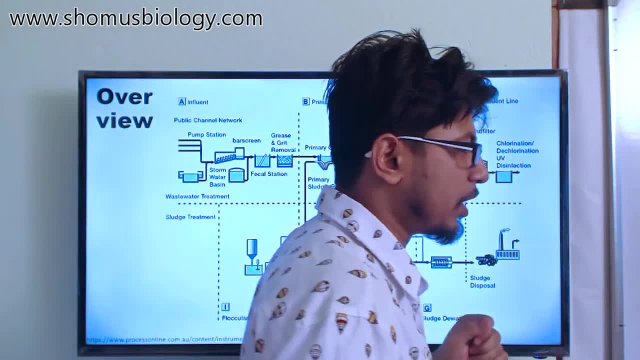 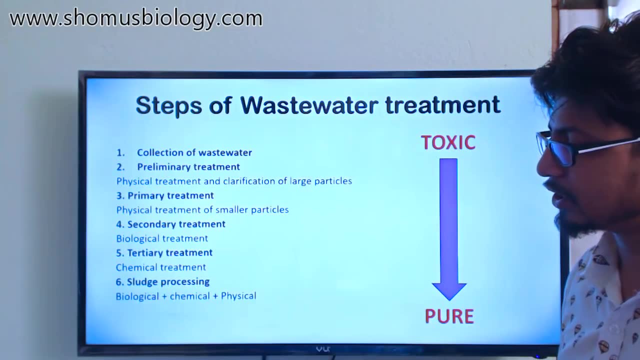 now, I hope, is crystal clear. so this is an overview of a wastewater treatment with all the seven different stages that we just talked about. so now in the series of video lectures we'll be talking about individuals. so this is in the first video. I just talked about the 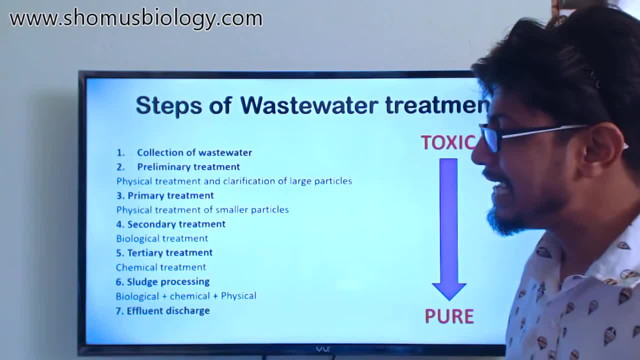 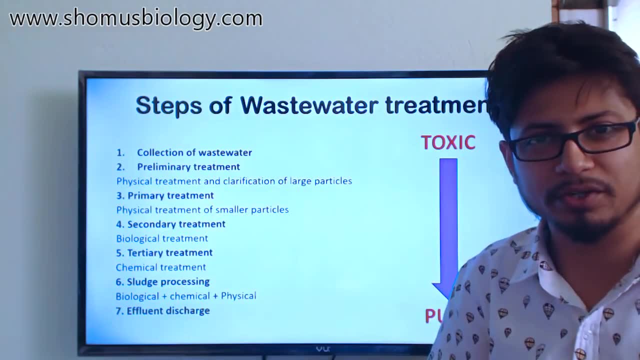 overview and I also talked about the preliminary treatment of wastewater. in the next video we'll talk about the primary treatment and then so on. in different set of videos we'll talk about different parts of this wastewater treatment. so keep on watching this video to understand the steps of the. 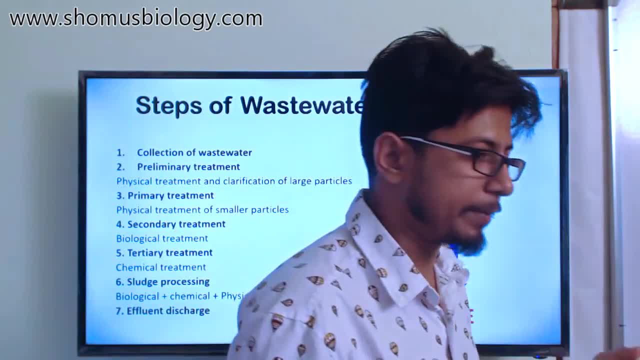 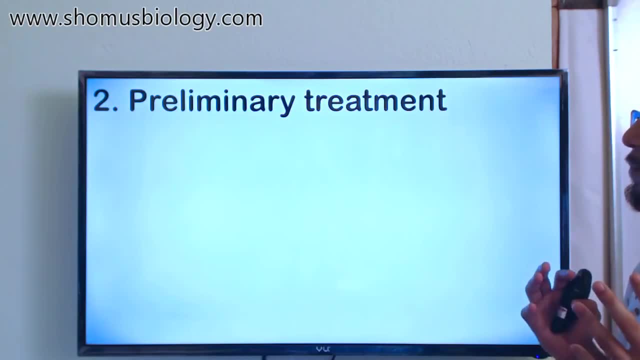 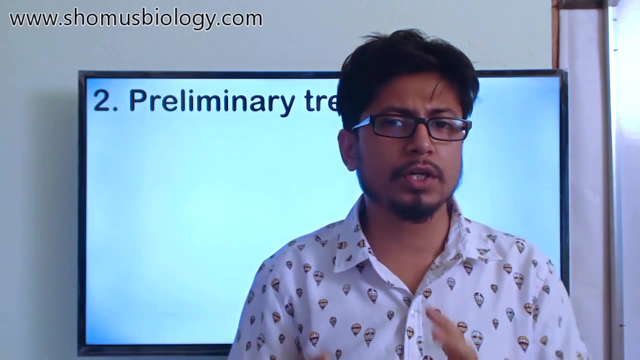 wastewater: treatment, processing and all the important steps, including the detail of views. so to summary up, we are going to talk about this preliminary treatment now. the preliminary treatment of wastewater depends on physical separation: physical separation of solids from the water and the solids generally. you know, because in 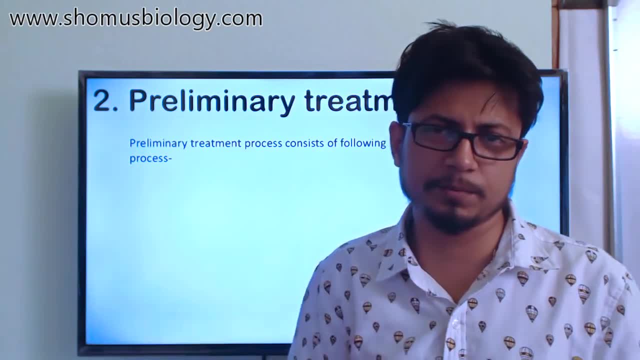 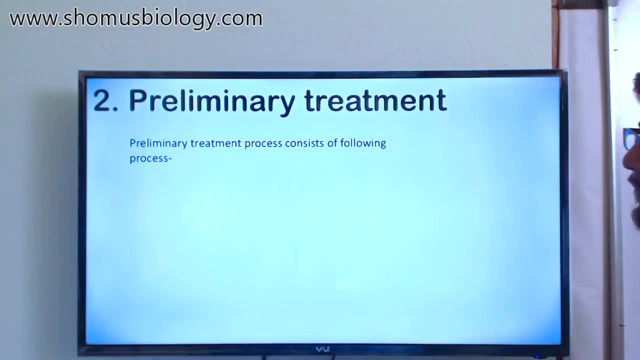 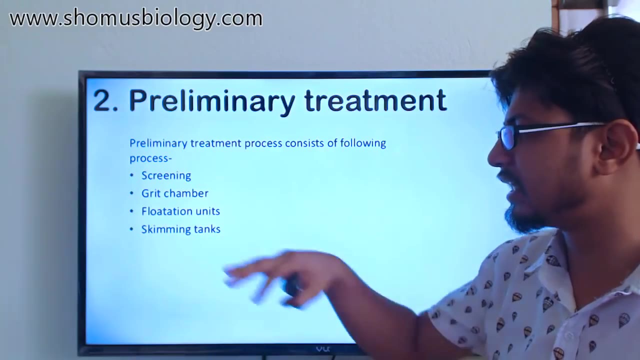 the sewage, in the water that we flush down, it contains many different solids because many different plastic materials, like you know, paper, papers and many more things that are present in there. so so in this preliminary treatment, we involve a screening, we involve grid chamber flocculation units and scheming tags, four different types of 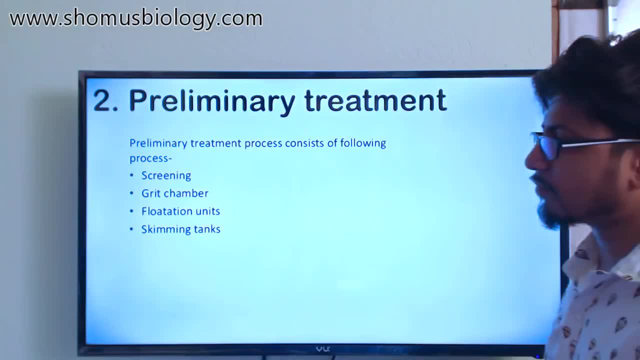 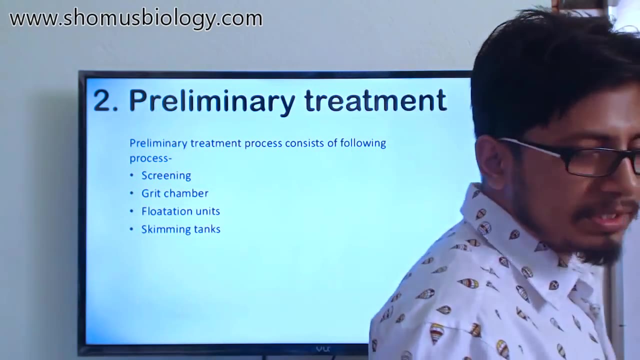 systems can be used. not a single wastewater treatment plant may have all. the four generally treatment plants can have one or two of this kind of treatment. generally, screening and grid chambers are the most common type of preliminary treatment, associated process and mechanism that we can use. one such example is shown in this picture. you 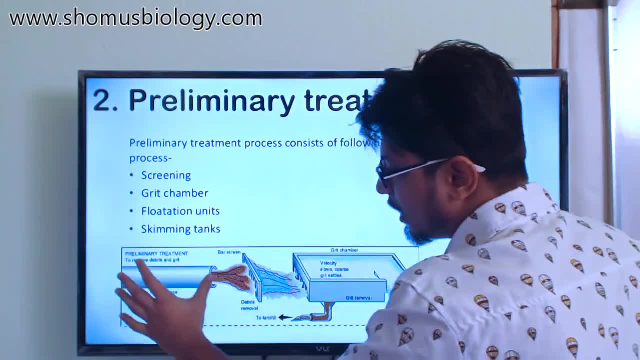 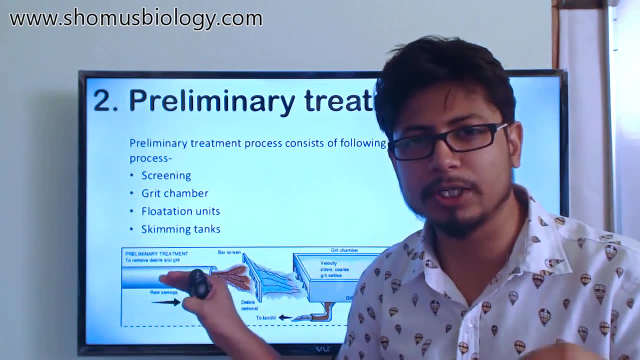 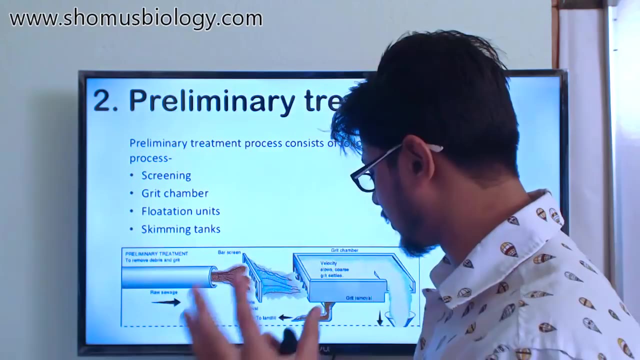 can see. this is from where the raw sewage is coming in. this is the collecting pipe. the collecting pipe, as I mentioned, huge collecting pipe, collecting all the sewage from every single household, and this is the most contaminated form of the water and you can see it filled. its color is given as brown. it's filled with organic matter, large particles, everything. 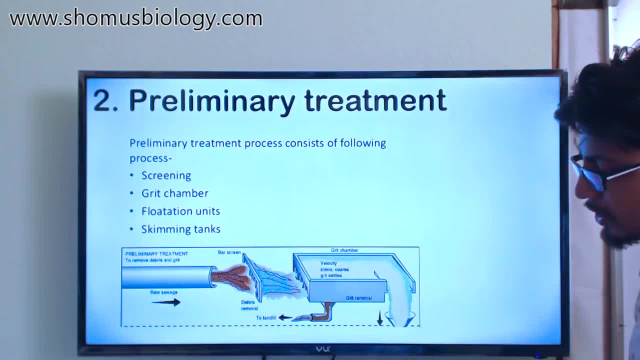 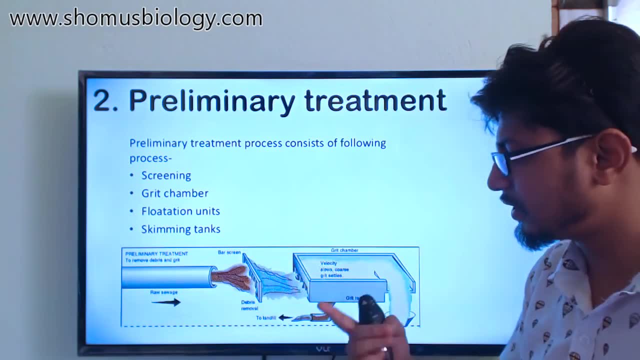 and these are the screens known as bar screeners. These bar screeners prevent the debris to move, So it's like a filter. it blocks all the large solid particles. So generally the bar screeners are like long bar, like structures like a grill that are present. 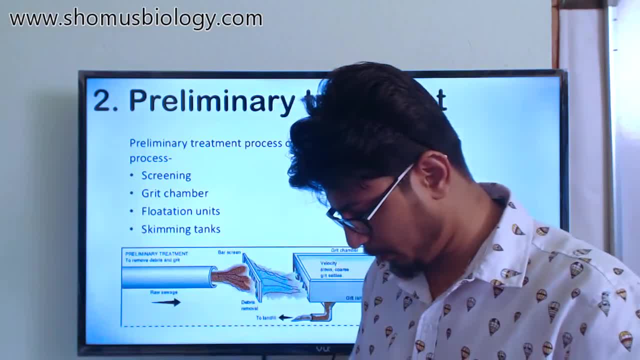 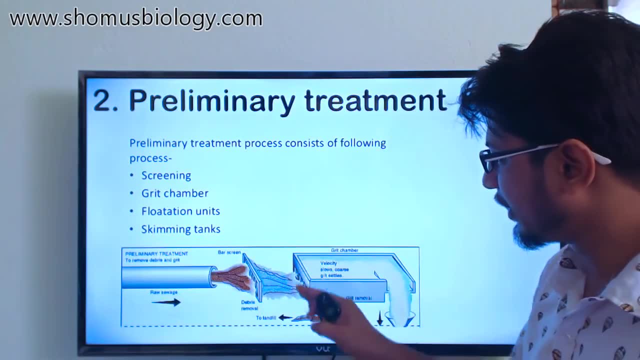 and in those grill the gap is like one centimeter to four centimeter. I mean one inch to four inch gap. that's possible and the debris are prevented. rest of the water flows inside the grit chamber. Now what happens in the grit chamber is that 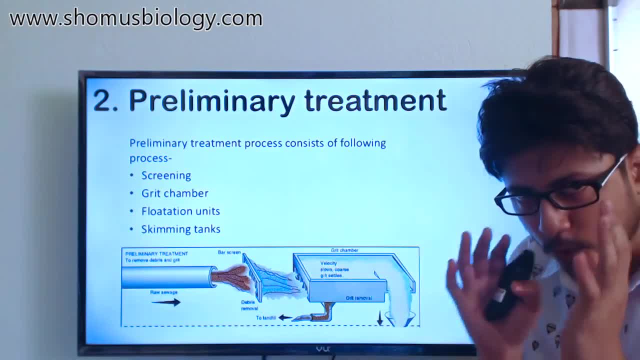 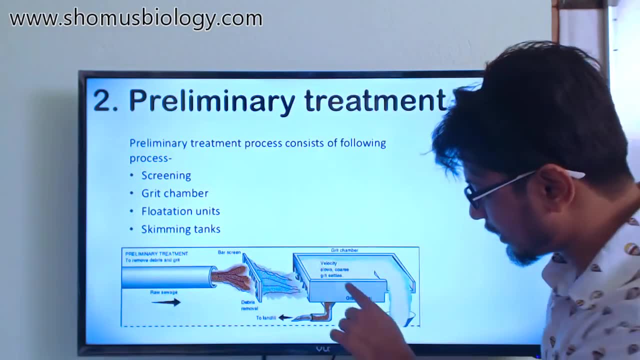 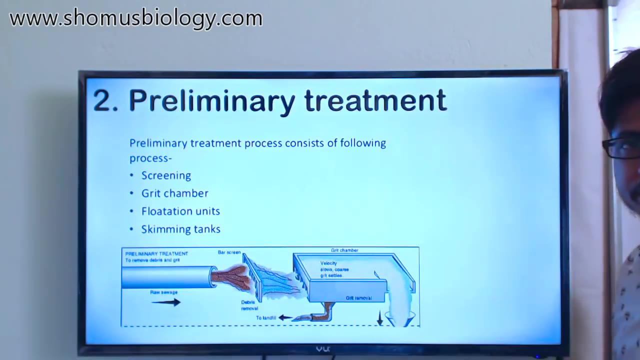 it's present in the grit chamber. So simply what we're doing is slowing down the flow. So in the grit chamber any other solid particles, they generally get settled down to the bottom. so we're just taking those grits that are settling into the bottle out and rest of the water is transferred from that grit chamber into the primary. 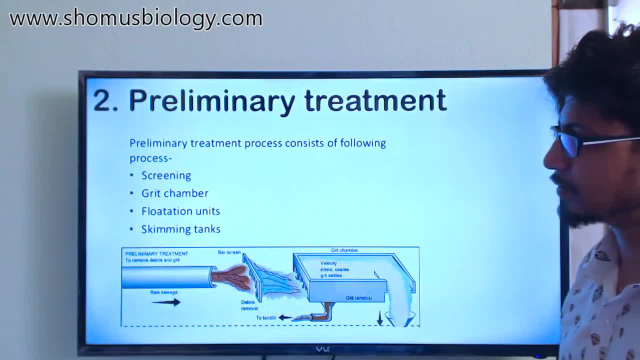 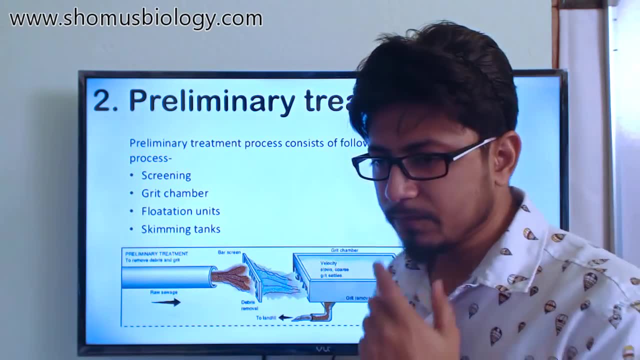 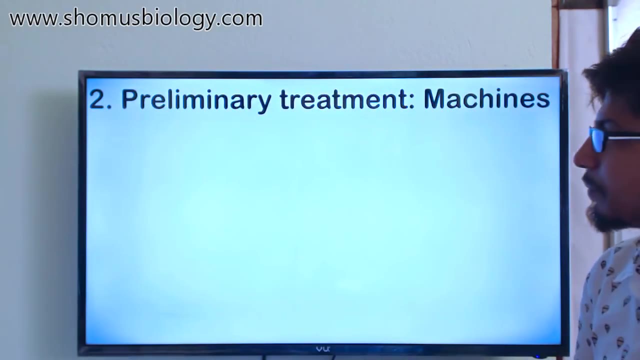 sedimentation tank or the primary system, primary treatment of this process. So this is what works in this process. So these large bars that's going to prevent this movement, And I'm going to show you these machines that are involved in the preliminary treatment. 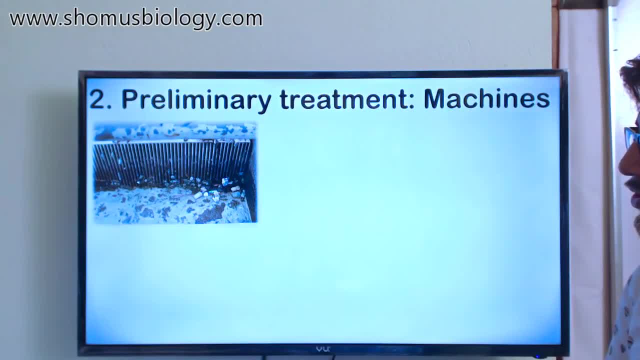 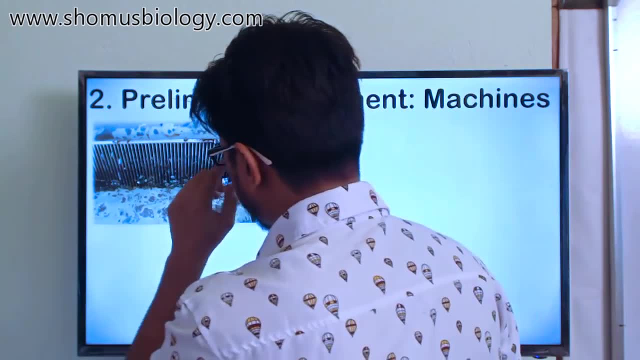 If you see- these are the bars or this you know screeners that are generally present- You can see, like grills, one to four inch gap between each of these bars And that's going to prevent a lot of bad material, a lot of large solid particles which are contaminating the water. 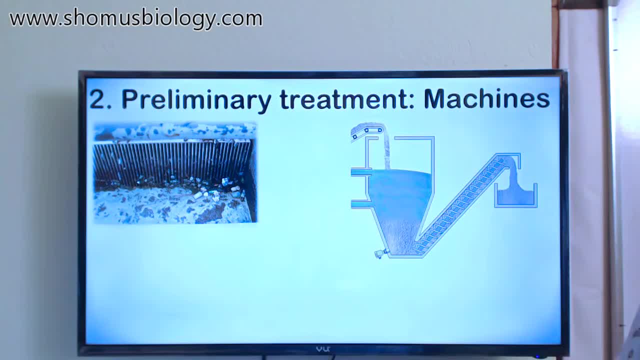 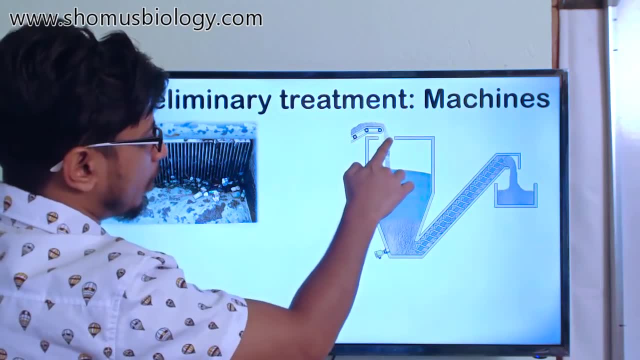 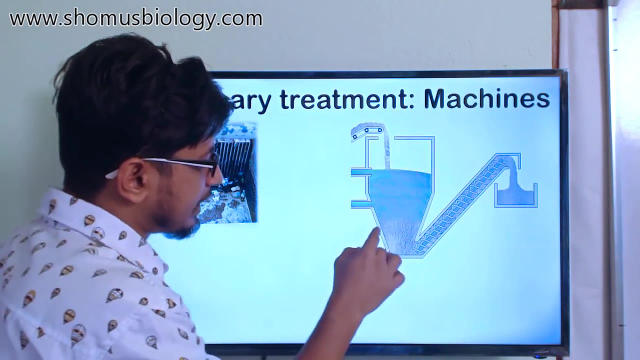 and the grit chamber. There's also another thing known as the grit washer. The grit washer works like a screw. As the screw is rotating, as you can see, there's a schematic drawing. This is where all the water, with the grits are actually falling, is pulled down to the large tank. in this tank you can see the 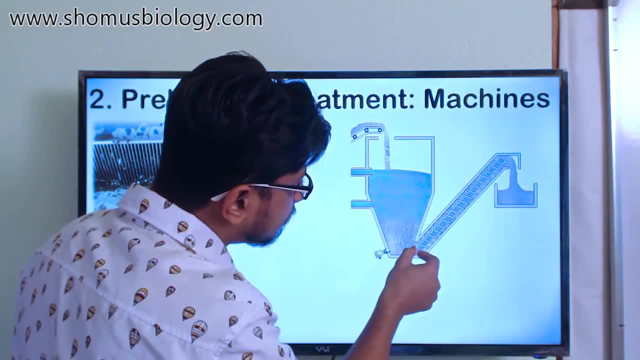 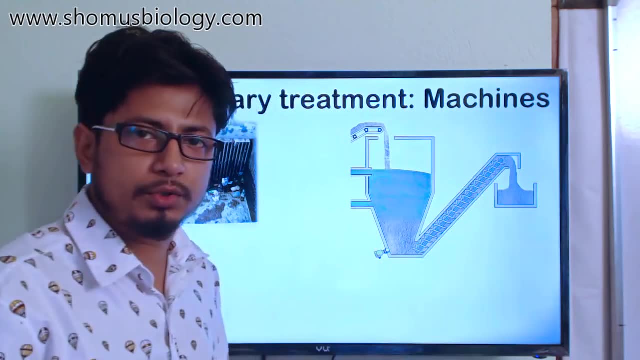 grease means the sonic particles are settling to the bottom and in the bottom it's a screw like structure connected and another chamber. this is a great collection chamber. so what this crew like structure is doing, it's keep on rotating as it's rotating is taking up all the great or certain solids to this. 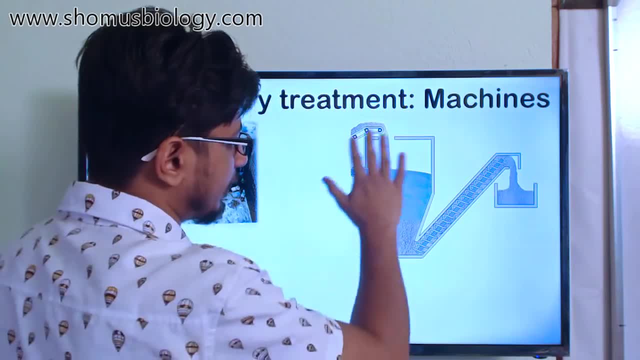 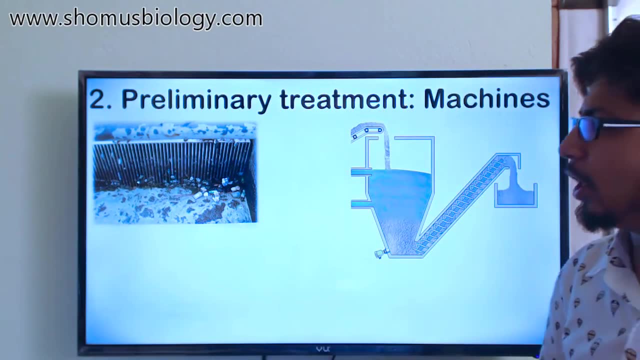 great chamber, and that's how the grid is separated from the rest of the water. so what we're trying to do in this picture, what we're trying to do in case of preliminary treatment, is simply to get rid of as much large solid particles as we can, because the more large particles we can get rid of, the better chance we. 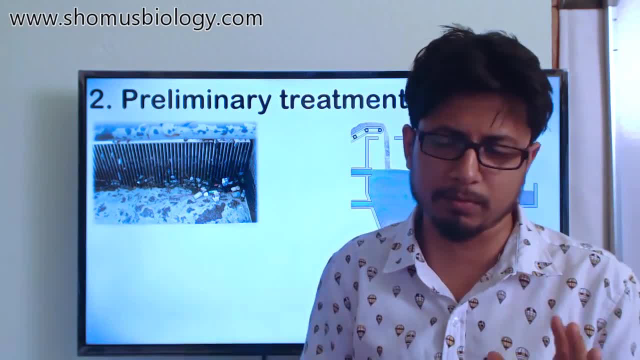 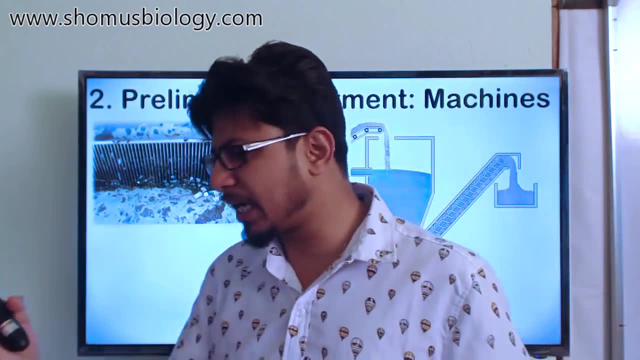 have to work with only water because you know, large particles create a lot of problems. we can which we can see from outside. so our job in the preliminary treatment simply to separate all the large particles which are kind of visible with our eye from outside in the water. so we are doing that. this is the 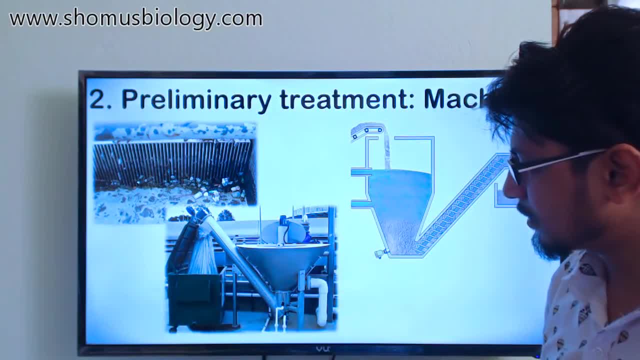 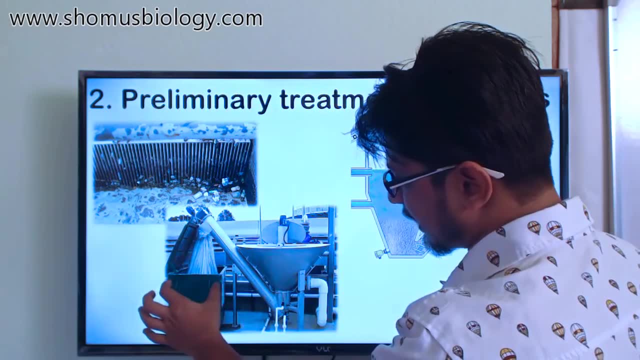 the, the, the, a realistic picture of, of a grid skewer or what we can see: the grid washer. this is the grid washer. this is the chamber where all the grids are stored, and this is like a dumpster and you can take this bin and we can throw that grid out. so this is one. 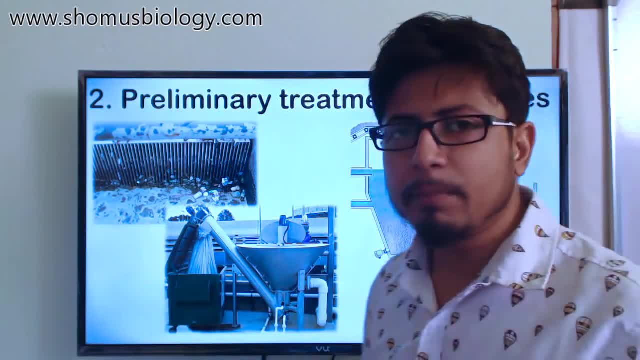 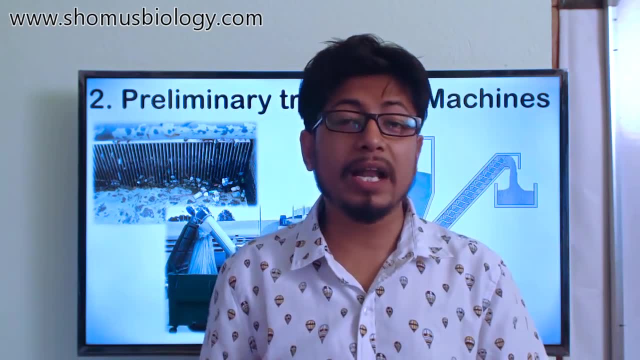 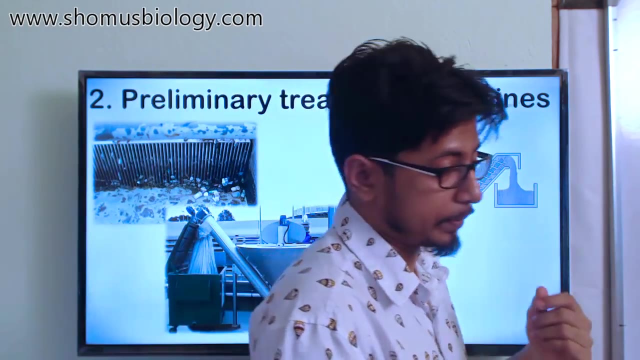 way of dealing with the large solids that are available. but preliminary treatment only continues to separate the large particles which are really really large enough to be separated, while in the primary wastewater treatment we'll see that very thin, very tiny in large small particles or solid particles can be separated because the 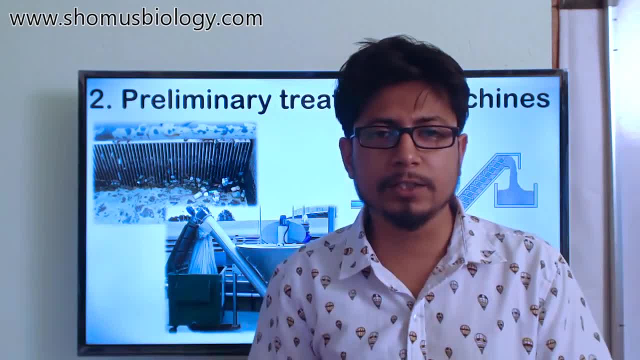 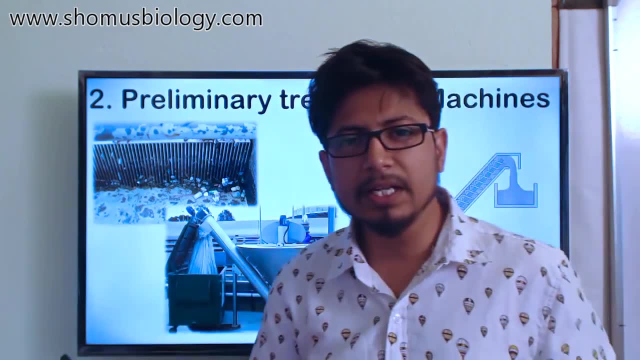 solid particles which are present in this wastewater can be large or can be very small. so here for very large particles may separating it with the help of the preliminary treatment, but with the help of primary treatment, will see we're separating smaller solid particles. so that's only the difference between. preliminary and primary wastewater treatment. another difference between preliminary and primary is that preliminary treatment we use hardcore physical separation, while in primary wastewater treatment mostly use the gravitational force and we reduce the flow of the water to separate the solids from the liquid. now let's talk about the 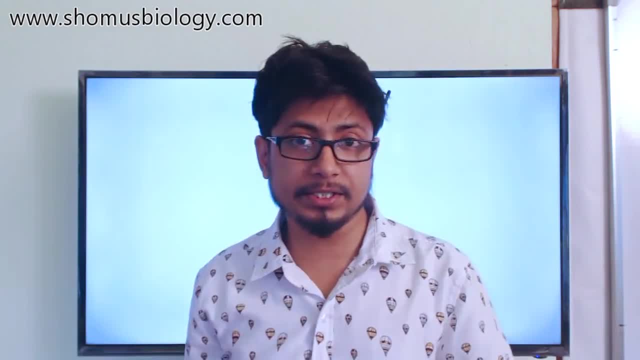 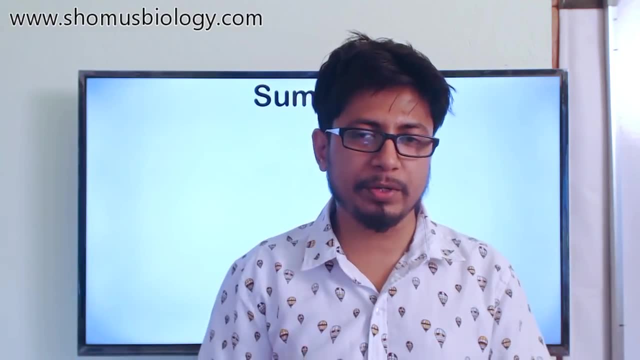 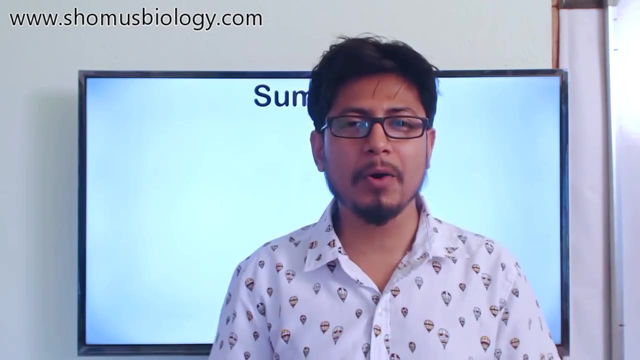 summary of all these wastewater treatment facility that we discussed. we've been talking about the wastewater treatment for a long time. we've seen the overview. we have talked about the preliminary wastewater treatment, the primary wastewater treatment, then the secondary wastewater treatment, then the tertiary wastewater treatment and now what happens after all this wastewater? 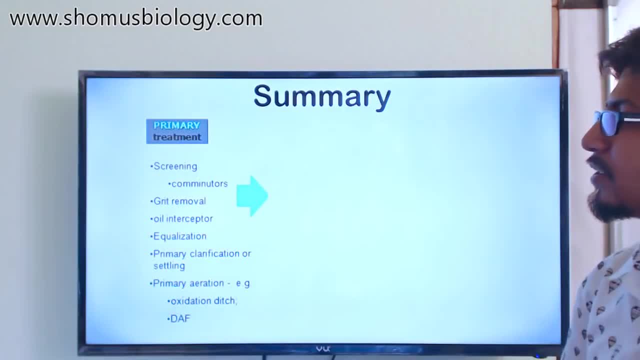 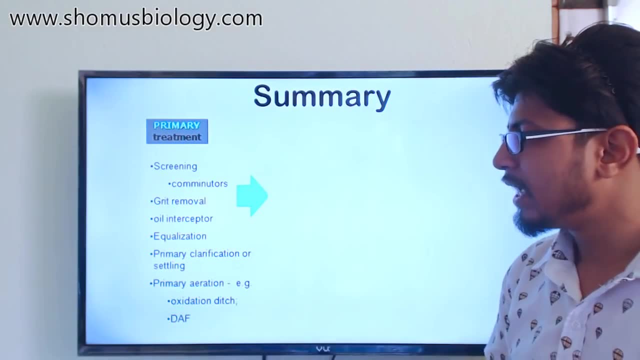 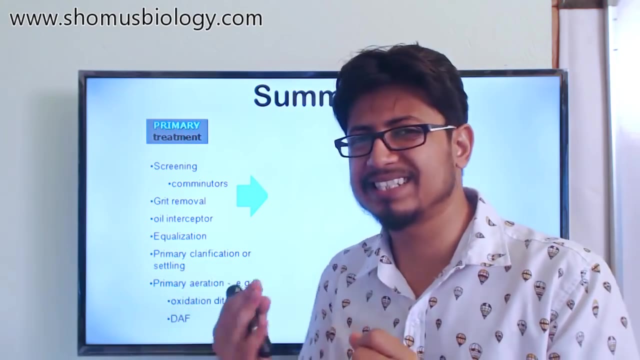 treatment modification. let's look at that in a primary wastewater treatment we simply use screeners- actually grid removal, removal of oil and primary clarification in the primary settlement tank- and we produce two types of solids. one is the scum which is present, like this oil components, on the top of the 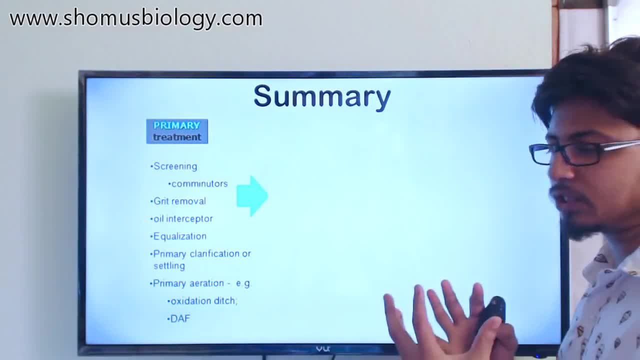 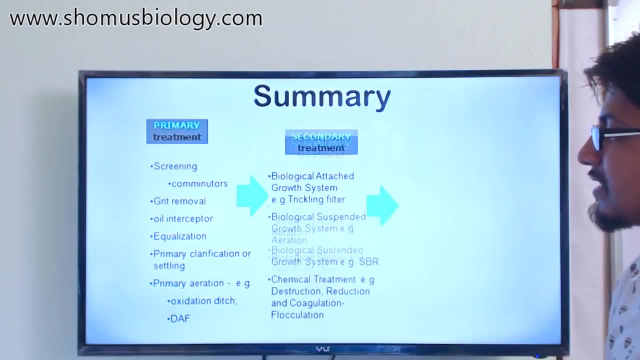 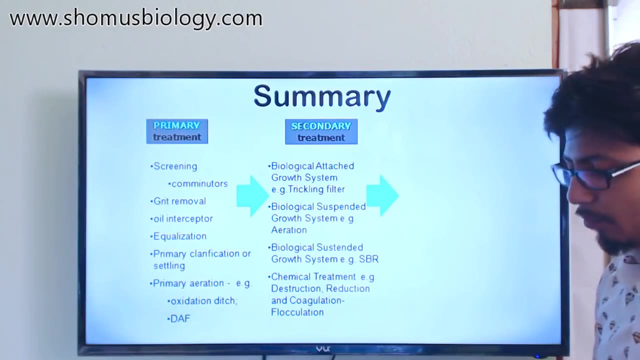 top layer of the settlement tank and we also produce large solids which are settled to the bottom, known as the sludge, and we then separate sludge and scum from the water. In the secondary wastewater treatment we use biological agents. either we can use submerged cultivation system or we 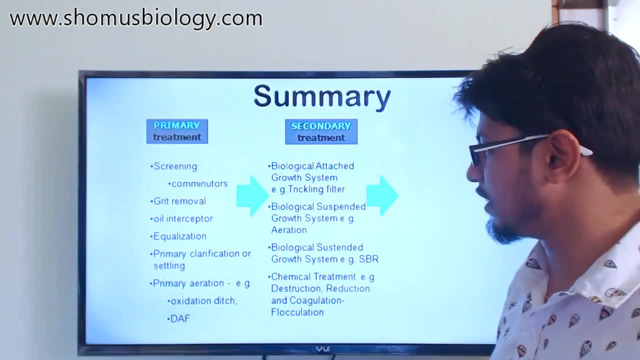 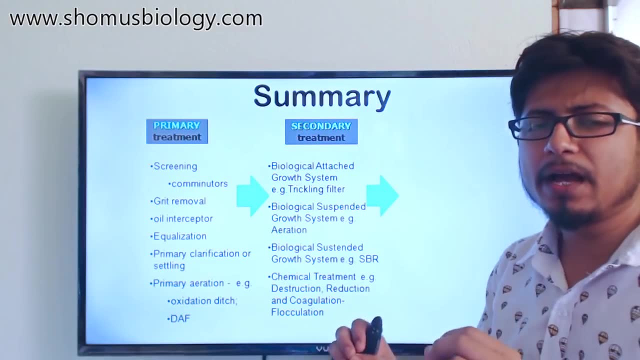 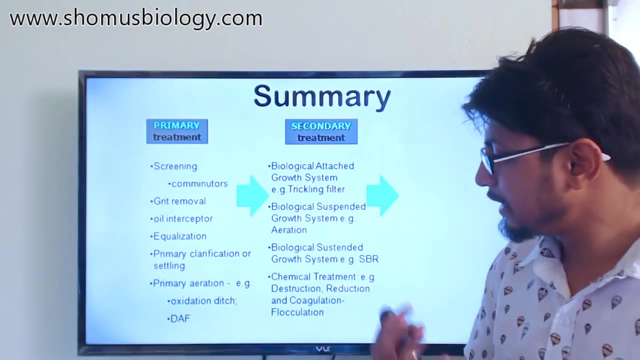 can use attached growth system, like trickling filter, and the suspended system like aeration- both the systems. but we use bacteria, fungi or protozoa to take up all the nutrients, like the organic compounds that are present in the wastewater, utilize them for their own group and producing the toxic debris. 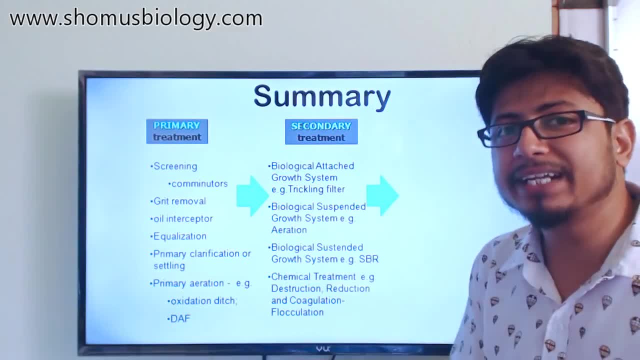 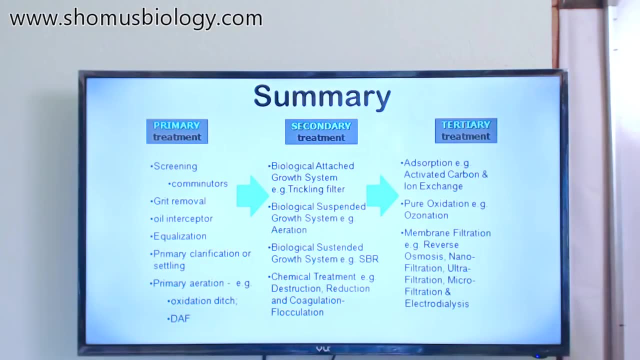 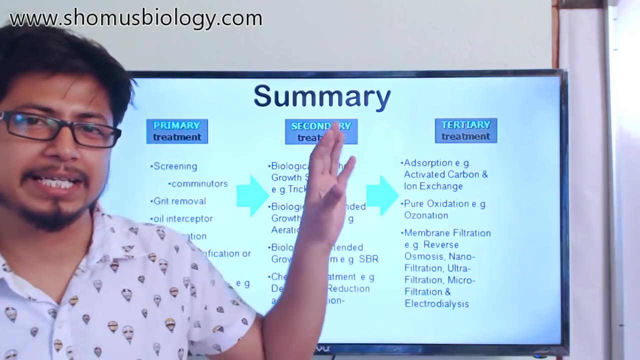 and materials which are also being settled down into the secondary sedimentation tank or secondary clarify tanks. okay, and then finally, in the tertiary wastewater treatment, we just take that water because we need to kill any other microorganisms that are present in that wastewater. after the secondary wastewater treatment: 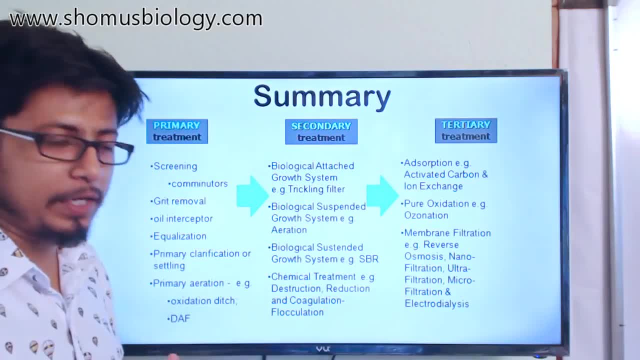 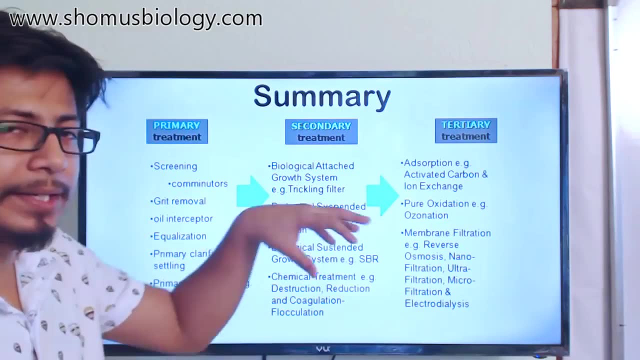 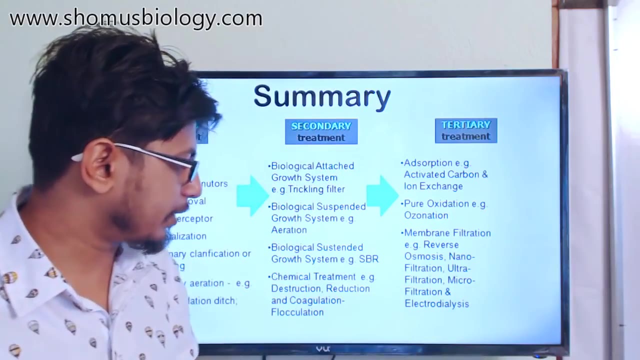 So I, we simply first use gravitational filter to separate all those bacteria, fungi, protozoa out of the effluent water and then we take that water and treat it with chlorine to kill any other chlorine or ozonization or any micro ultra filtration- micro filtration, okay- or reverse osmosis type of processes to get. 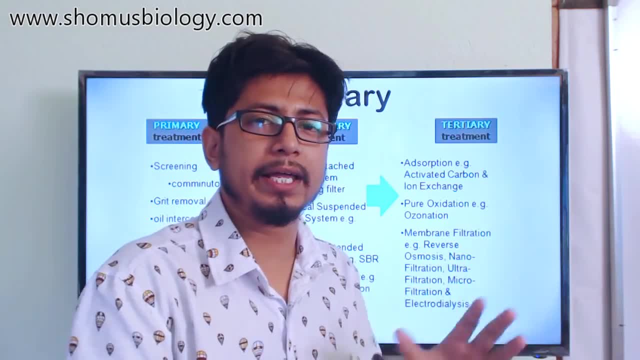 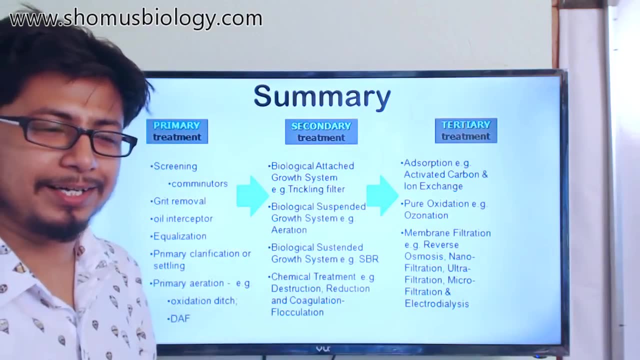 rid of any other chemical components, heavy metals and any microorganisms to be present there. so we get rid of all of it at the end of this tertiary treatment and then we release the effluent to the discharge facility. okay, so these are the steps the primary treatment deals with.